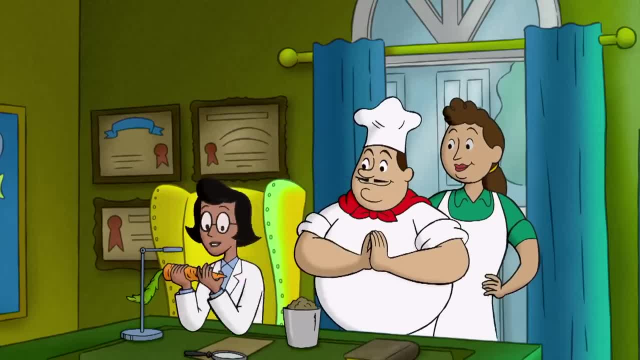 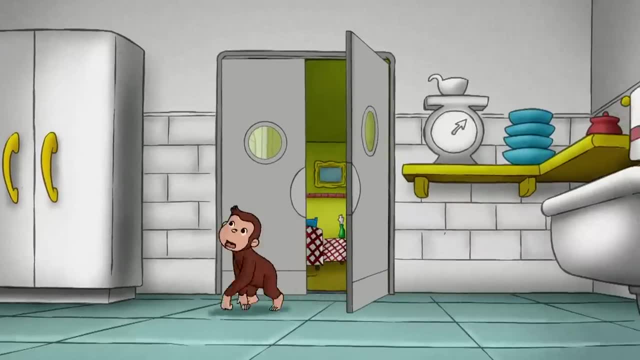 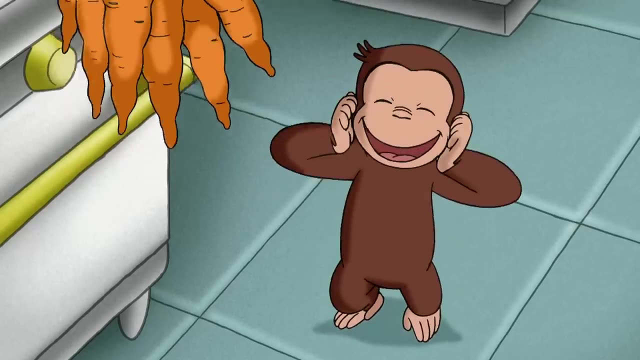 Okay, I'll run tests. Can I keep the carrot? Nope, sorry, I'm making soup. Oh, George. Hey, look at the carrots we planted Already grown. huh, You know, as long as I have my fresh veggies, I won't have to close down. 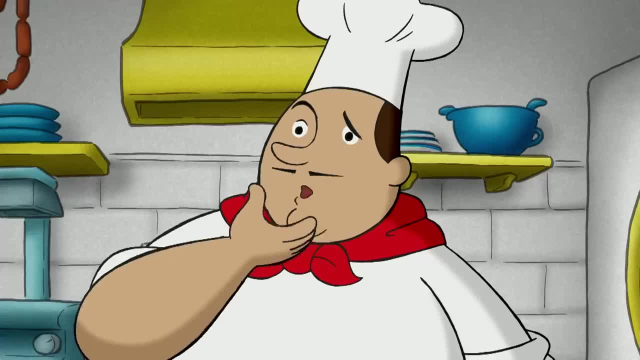 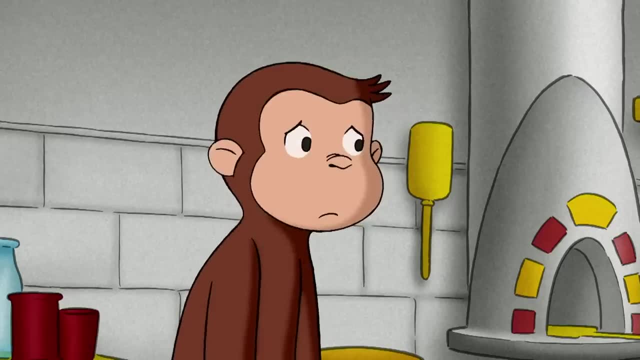 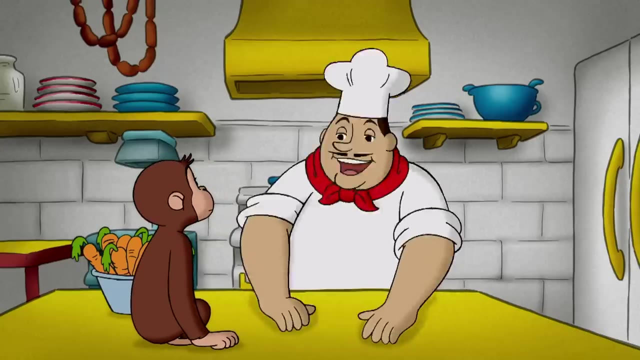 George felt like he'd made a good elf, But I wonder why the eggplants and squash did not grow. Oh, he'd forgotten the eggplants and squash. Later I'm going to plant those. If it works again, tomorrow we'll have peas and arugula. 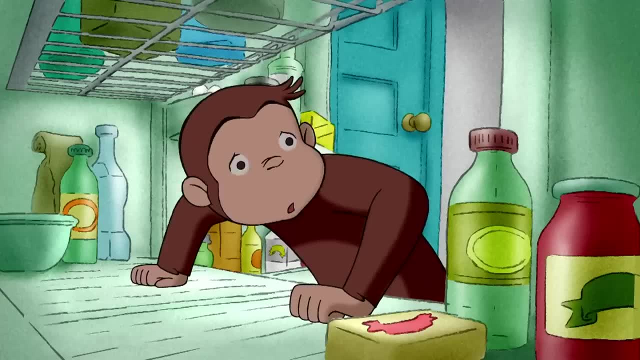 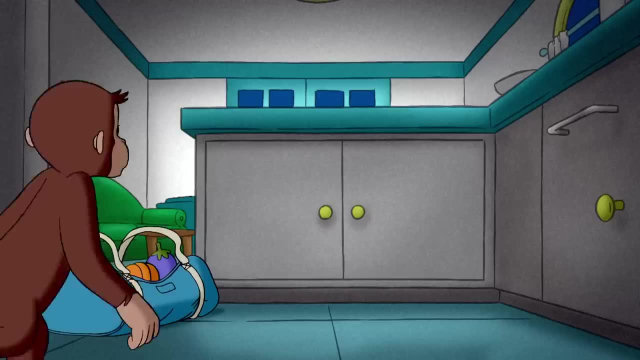 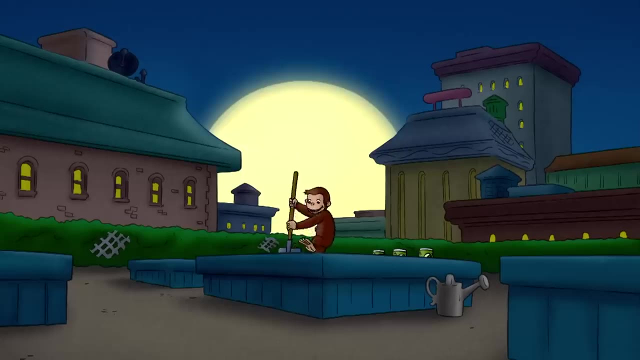 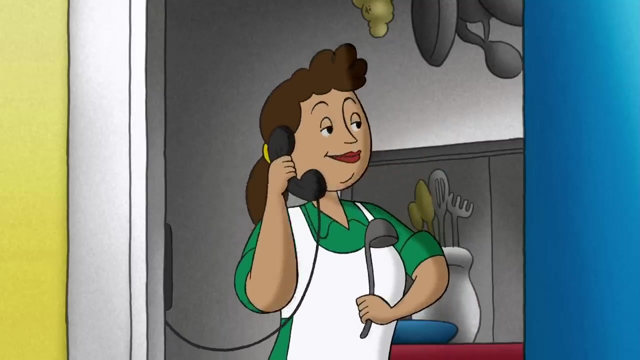 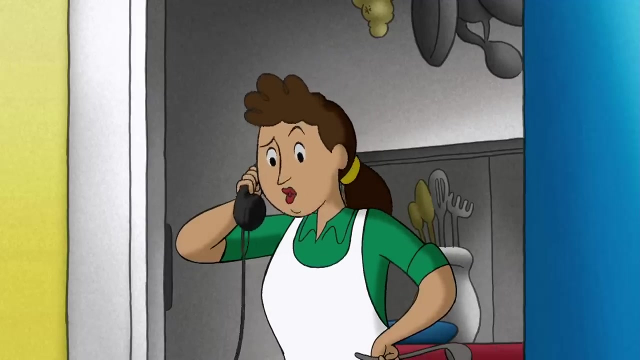 Eggplant Squash, But where were peas and arugula? How could George be an elf without fresh vegetables? Okay, Ah, hello, Professor Wiseman, Our dirt is just normal dirt. No, I don't know yet if it happened again. 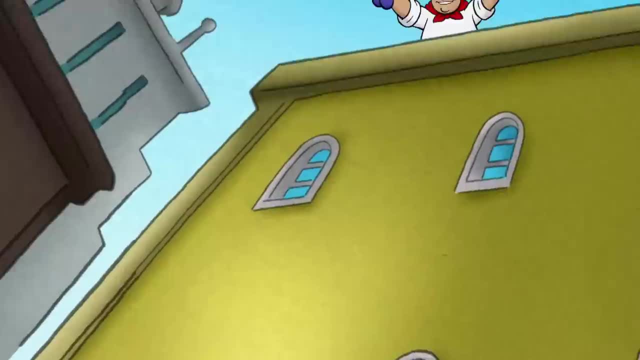 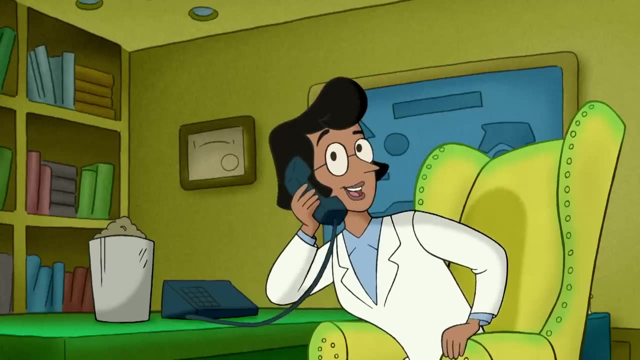 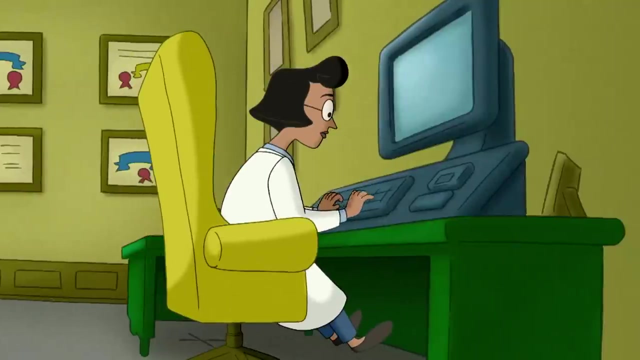 And it's happened again. We got eggplant. We got squash. Come and see, Ah, Squash, Eggplant. I'm coming right over. Don't Make Soup Einstein Pizza. Meet me at Piscetti's Stat. 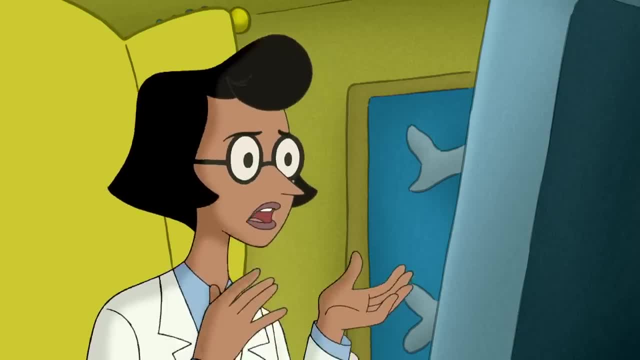 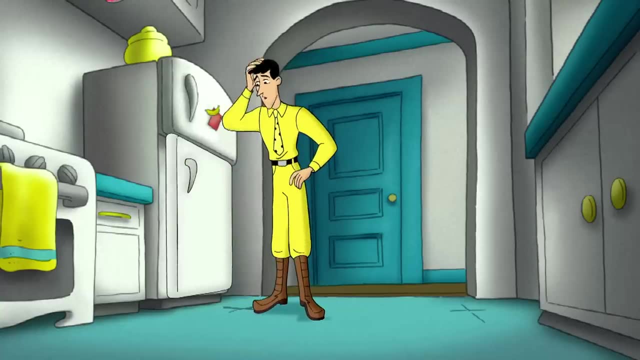 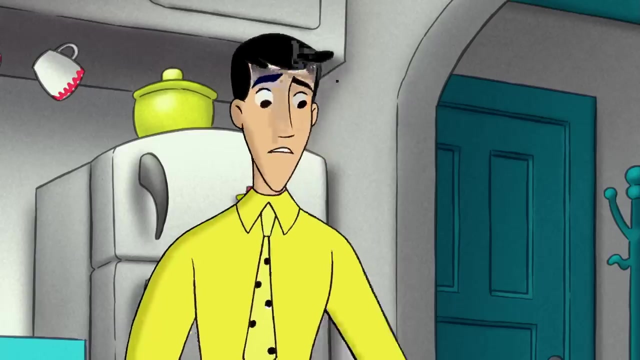 Are you buying? We're not eating. We're being scientists. Uh, George, Did you, um, do something, which I don't know what it would possibly be, with all of our vegetables? Uh-huh, You're feeding a vegetarian cobbler. 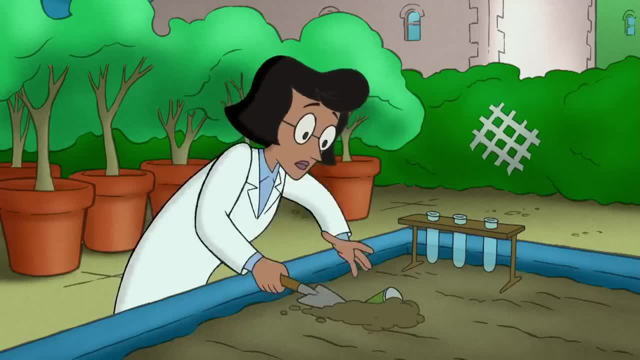 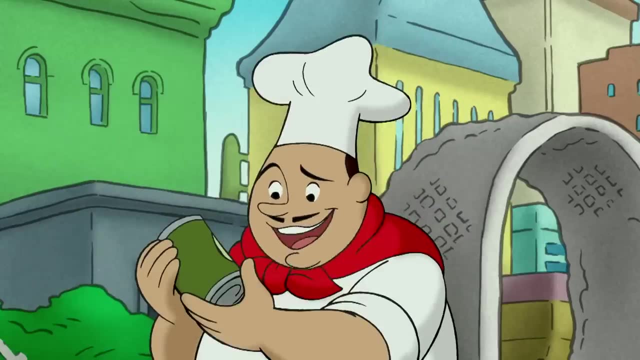 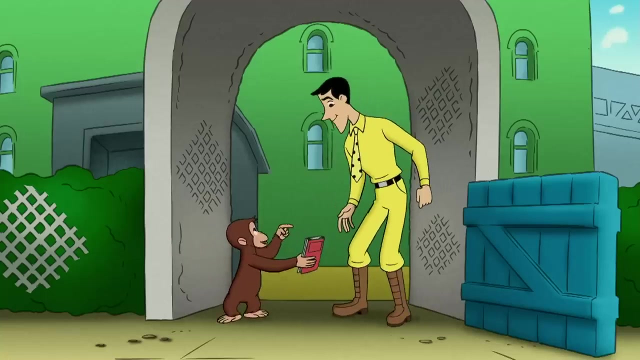 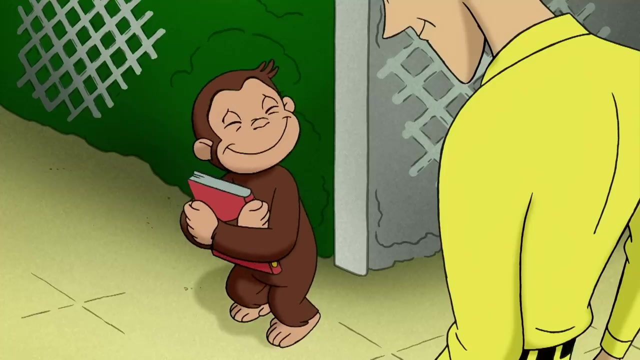 Hmm, Did you plant a can of peas? They're growing in cans now Natty, call the TV news. Oh, how they're facing there. Oh, wow, wow, wow, Uh-huh, Oh boy, Oh hi everybody. 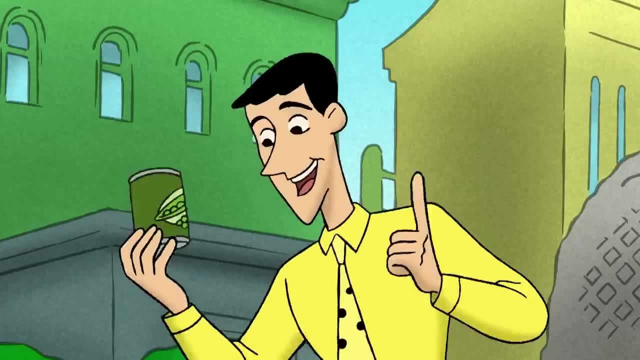 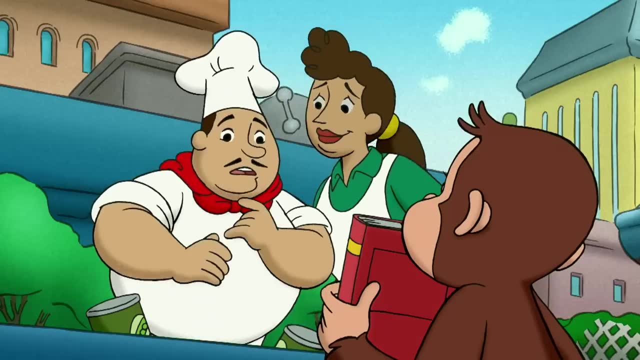 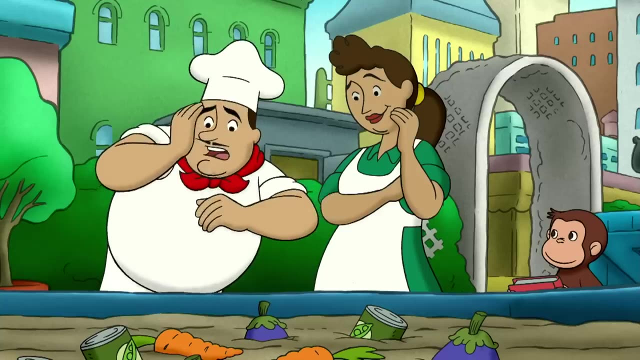 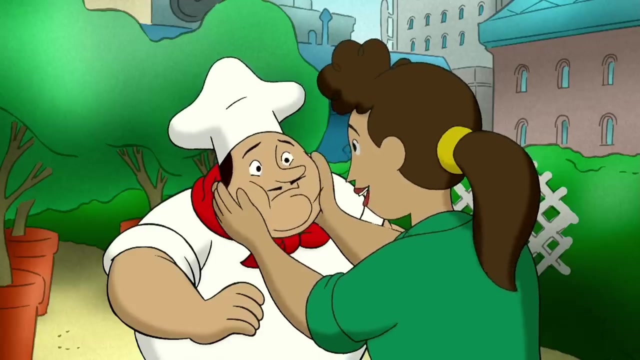 Well, um, this would be mine. You see, George, um wanted to be your elf. Oh, you did this, so my garden would grow fast. Uh-huh, Oh Natty, our garden is not magic. Ah, but your cooking still is. 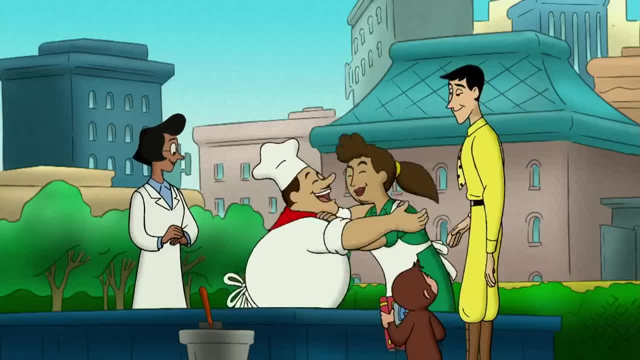 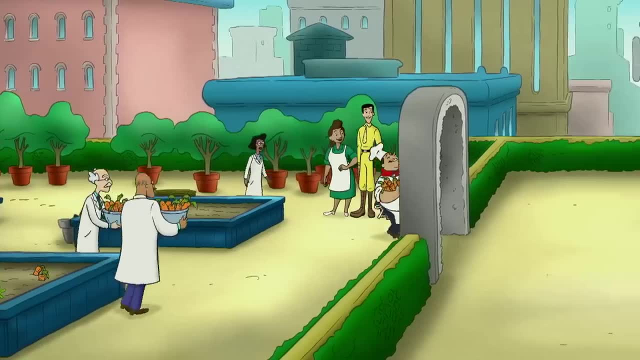 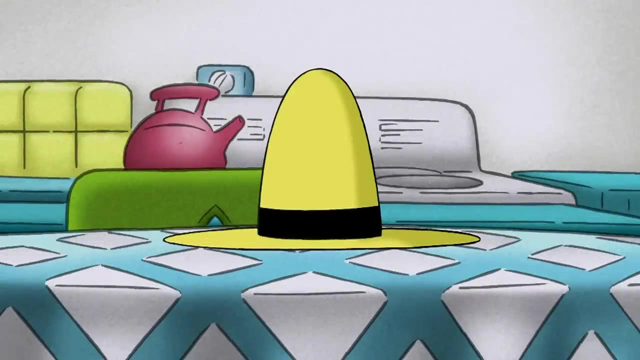 Well, you got me there. That's right. I'm great. I'm gonna cook all these veggies up as lunch for everybody. Come on, I'm hungry. The man with the yellow hat's hat was special, But what made it so special? 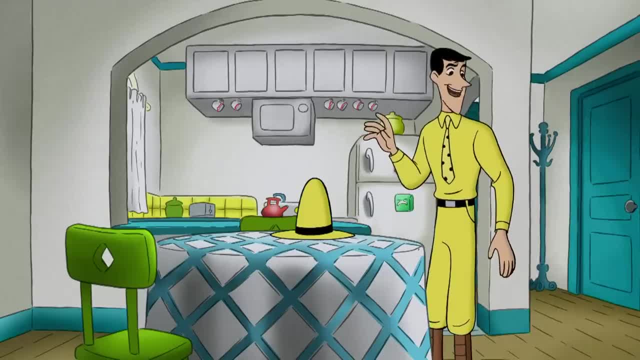 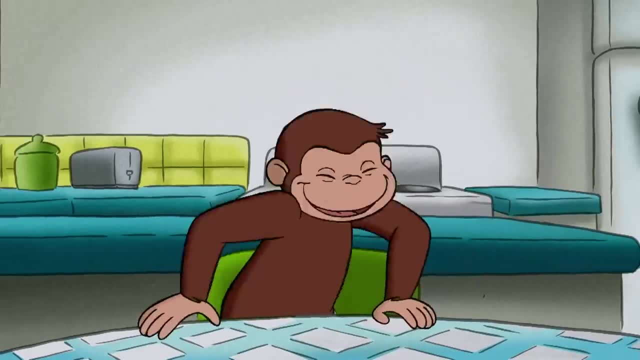 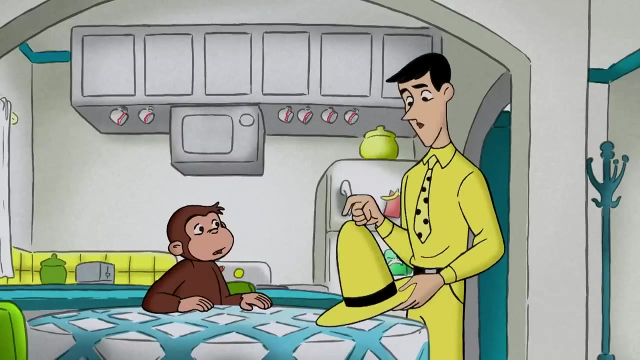 George, come on, It's time to go. When I put my hat on, I'm all ready to head out the door. What Huh, What? Okay, George, that was funny, but you know the rule: No one is allowed to play with the yellow hat. 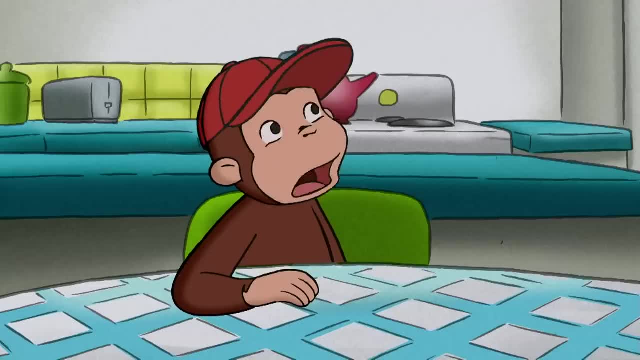 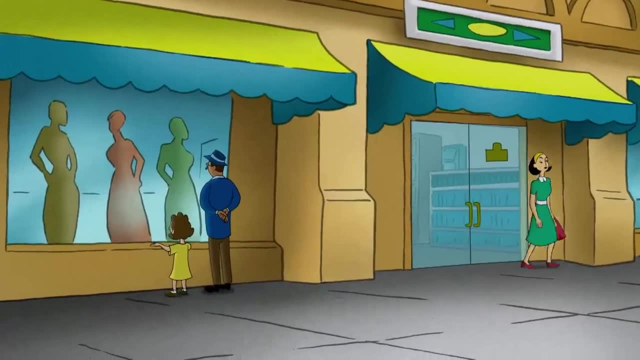 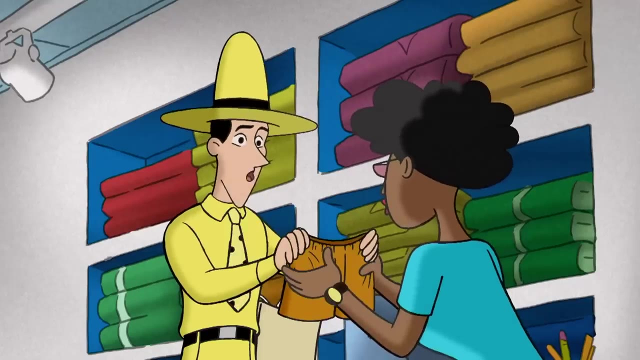 George sure liked that yellow hat. George's cap just wasn't special. I'd like to return these. They were yellow, but after only one washing they turned saffron. I have to make a big speech and I need to know my shorts are yellow. 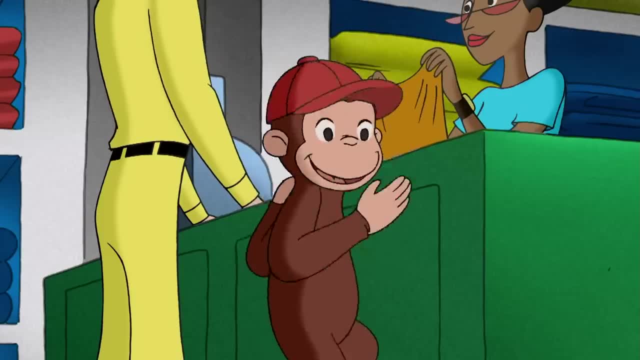 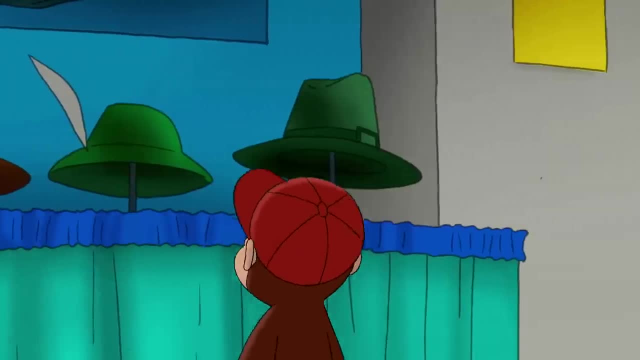 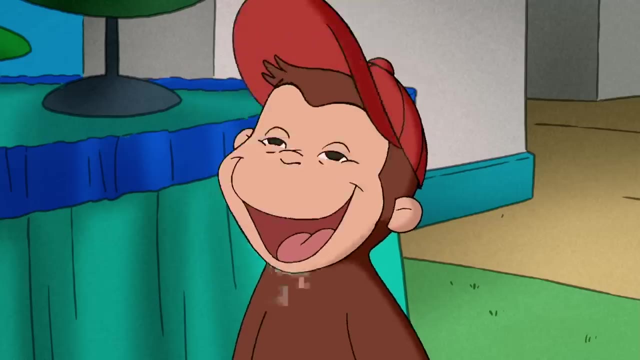 Oh, Ah, Hey, Oh, Oh, Oh, Oh. Like a hat of your own, George, Ooh, Ah ha. Well, which hat do you like? George wanted a big yellow hat, but there was only one of those in the world. 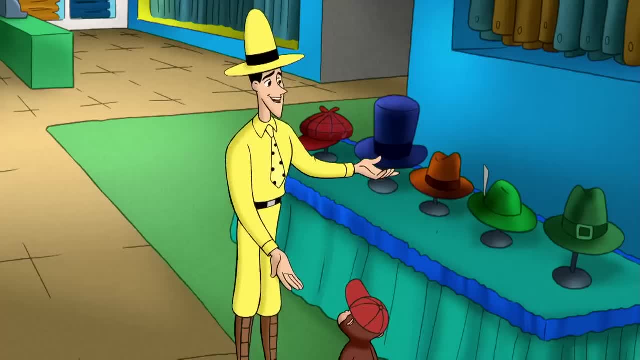 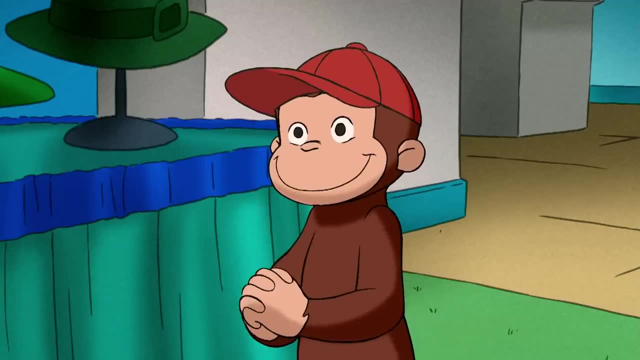 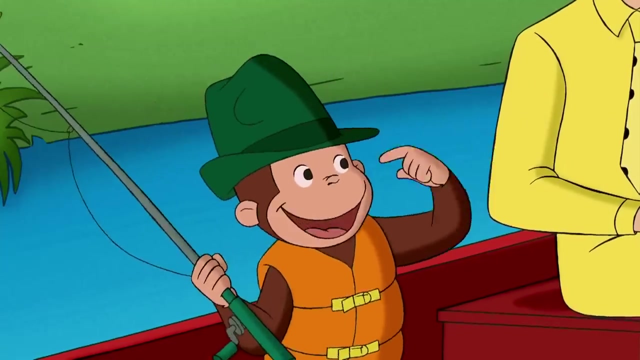 Well, you could try different hats till you find what feels right for you. So George began his quest for headgear. Hey, Where's George today? Huh Huh, Didn't recognize. ya, That's not a city kid hat. 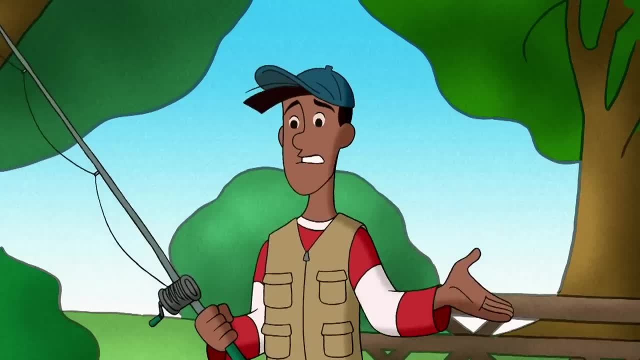 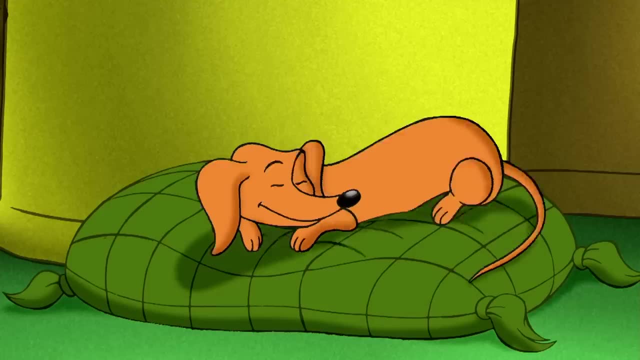 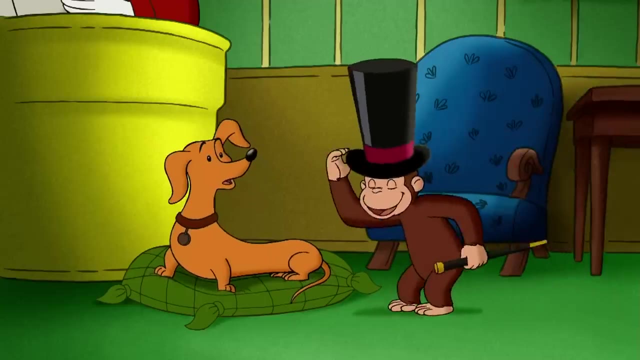 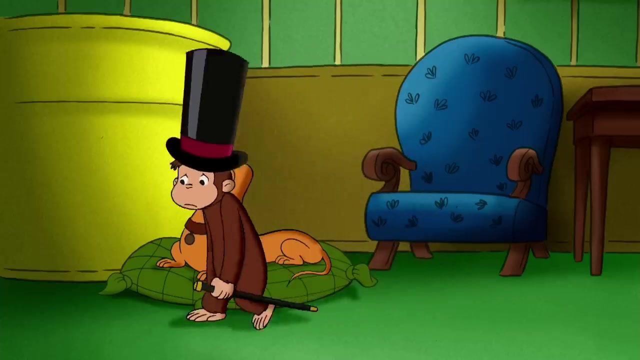 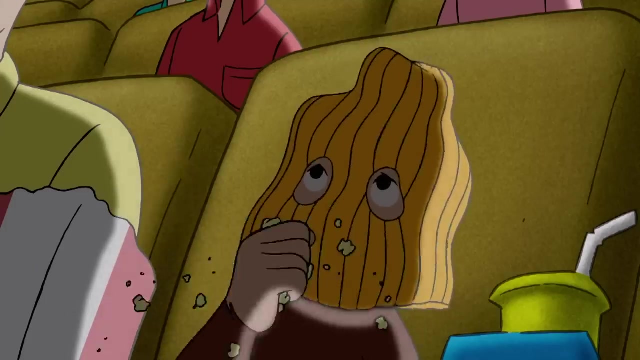 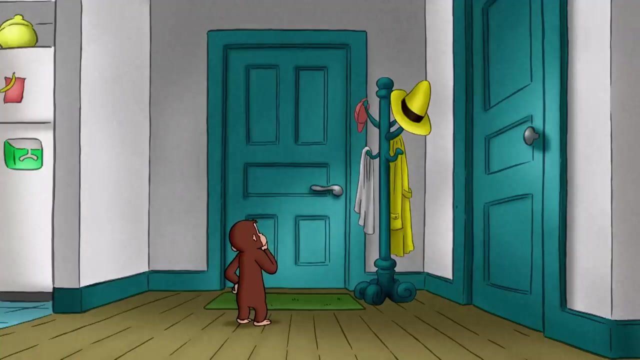 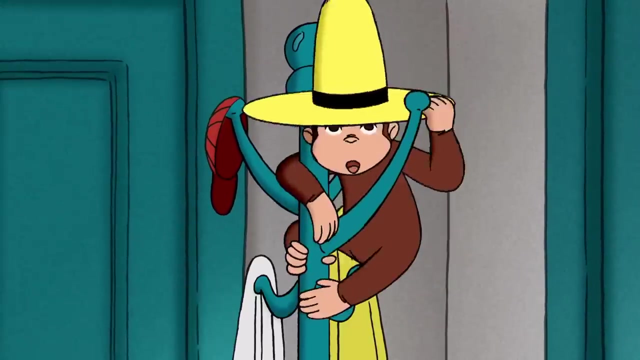 Some hats are right for some people and some aren't. Oh Ah, George's friends didn't appreciate any of his headgear. Picking the right headgear was not easy. What made the yellow hat so great? Ooh Ha, ha ha. 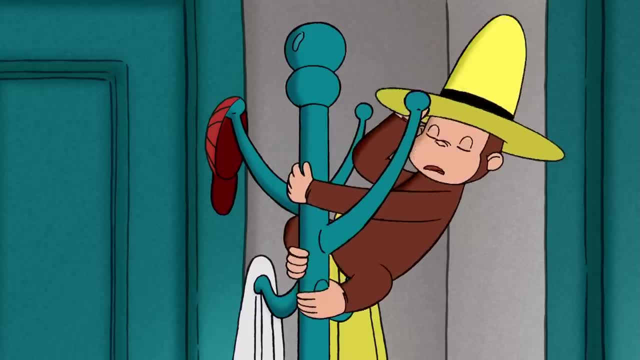 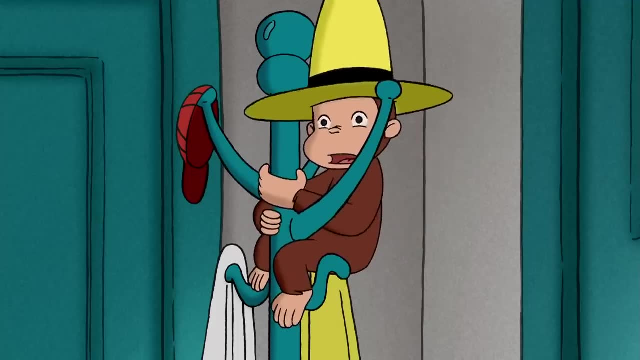 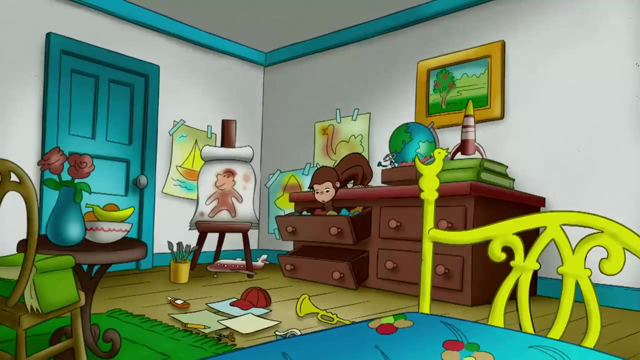 It was just plain fun. George, I need to wear the hat. I need to wear the hat for an important speech at the museum. Please don't play with it, Ah ha. That's what George wanted: A fun hat that he could play with. 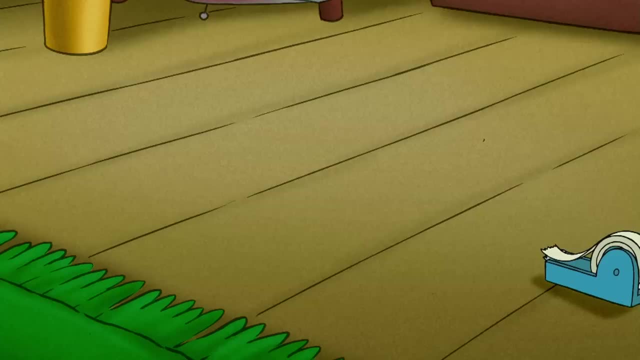 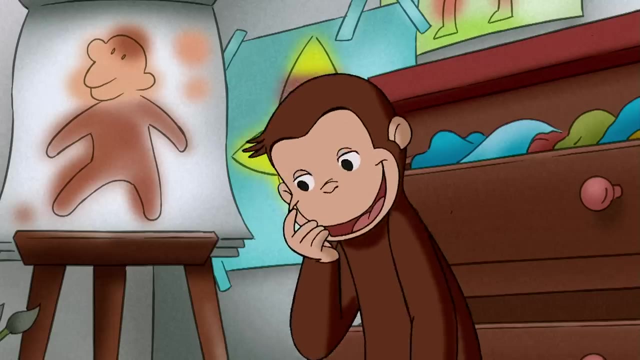 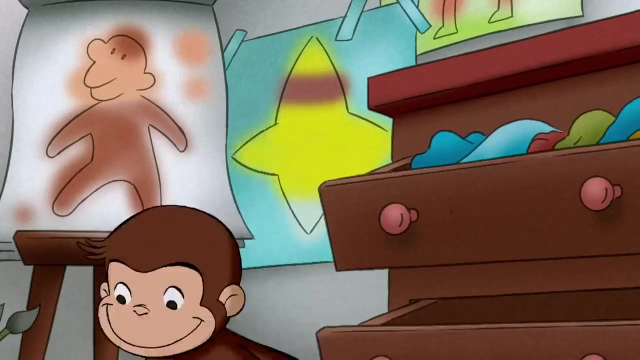 Ho, ho, ho ha ha, Mm, Mm-hmm, Ho, ho, ho, ha ha, Ooh Ha. George wanted his fun hat to be more than just a normal hat. He'd use his cap for shape. Ah ha, He would need an opening. 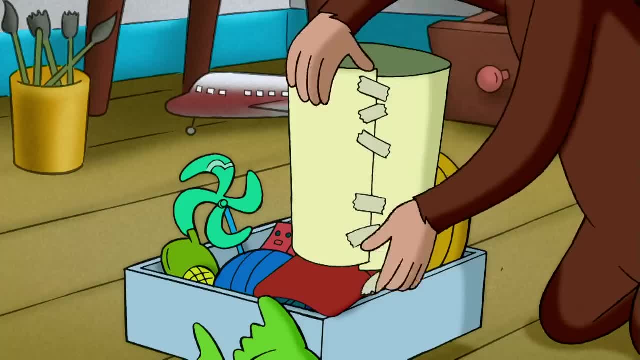 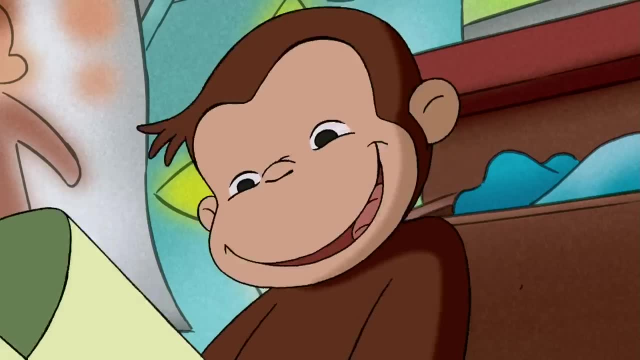 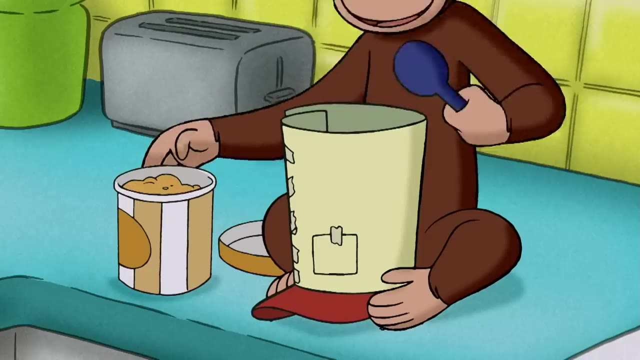 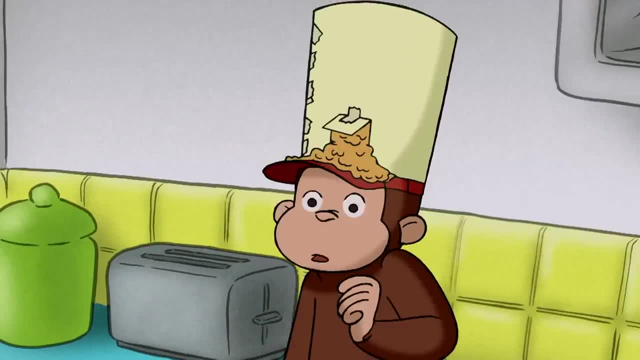 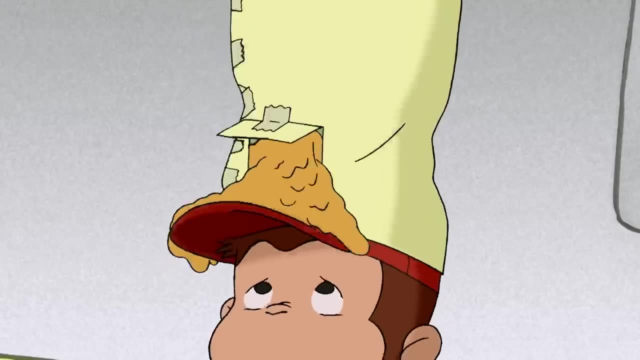 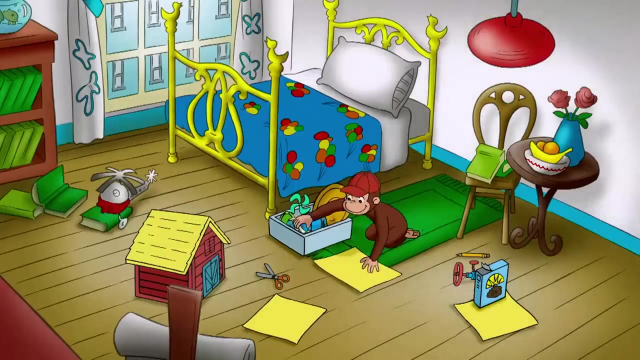 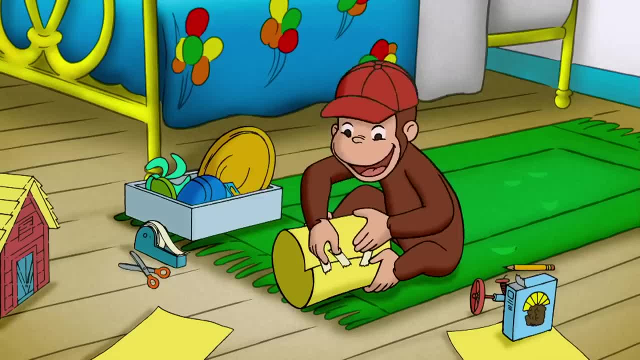 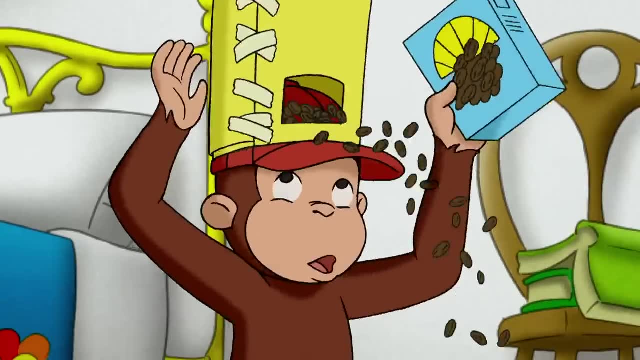 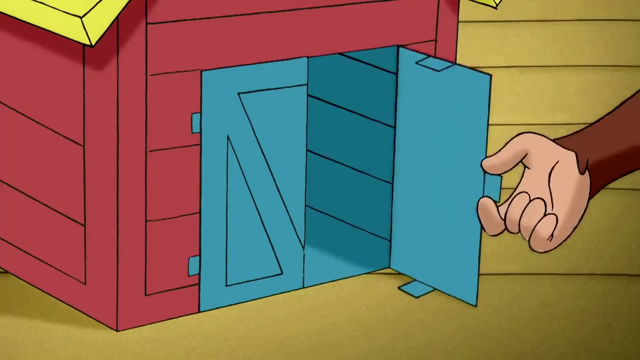 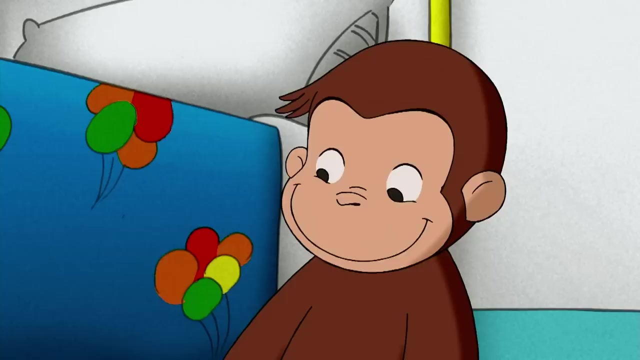 Ha, Ha, Ha, Ha, Ha Ha. And raisins instead of ice cream for a fun, healthy snack and a hat Oo hoo, Hmm, Hmm, Hmm, Ah, Pizza, Look at it, Mm-hmm. 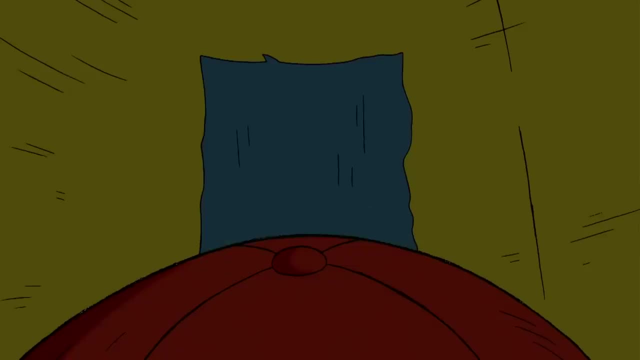 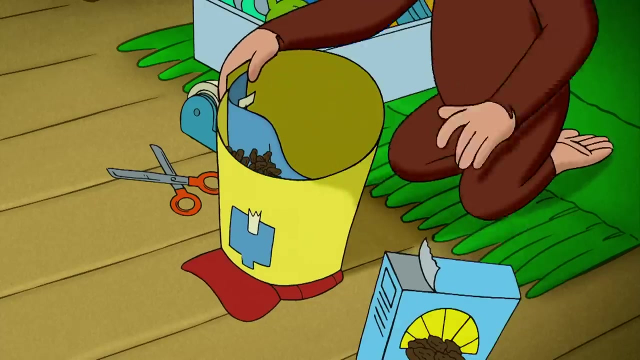 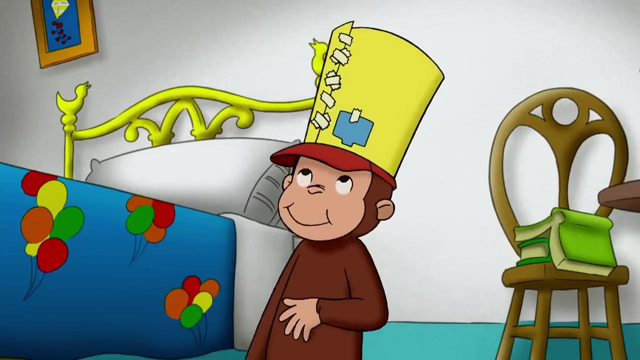 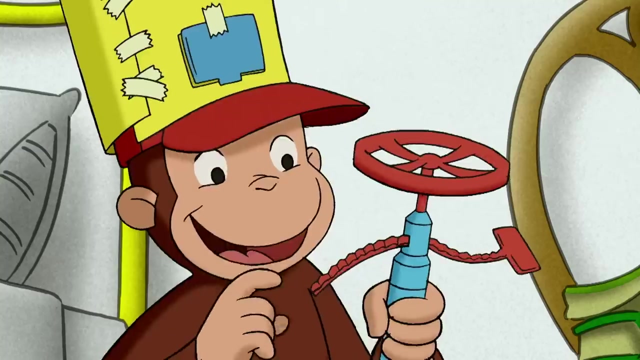 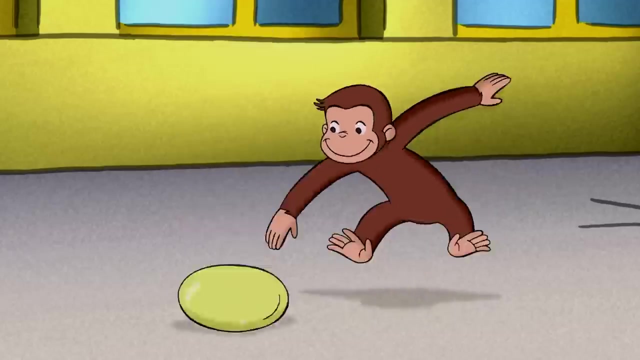 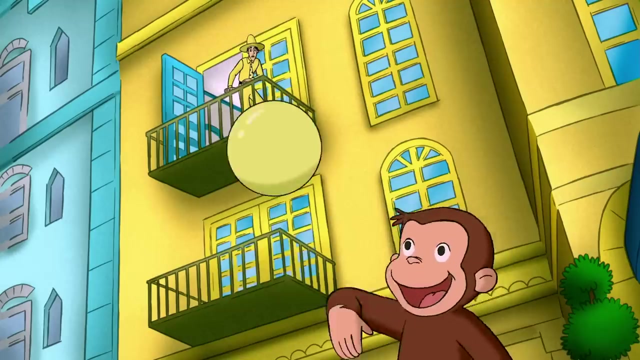 Oh, Oh, Ah, Ah, Ah, Ah, Ah, Ah, Hmm, Hmm, Ah, Ah, Spring had arrived. It was the perfect day for George to break his moon ball record. George Time to come in, Hmm. 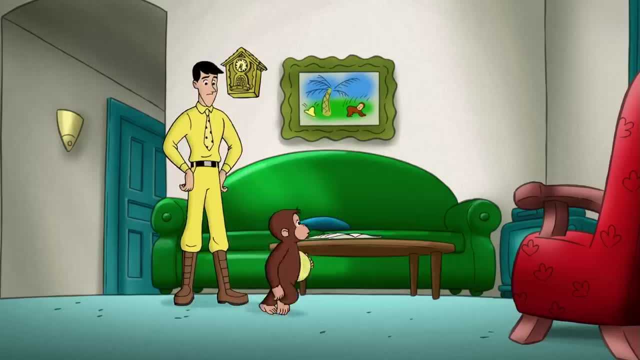 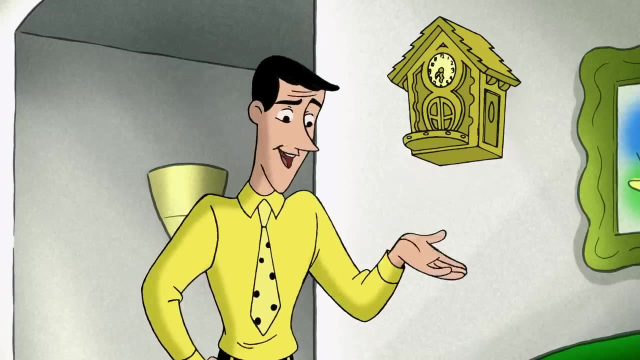 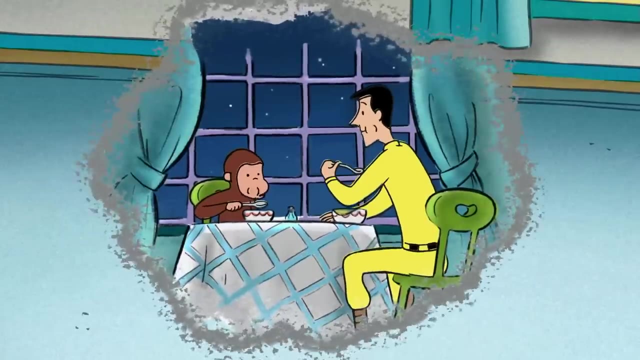 Come on Bedtime. Oh, I get it, You think. because the sun is out, you should be out. Well, George, in the winter the days are short, so it's dark at dinnertime and dark at bedtime. 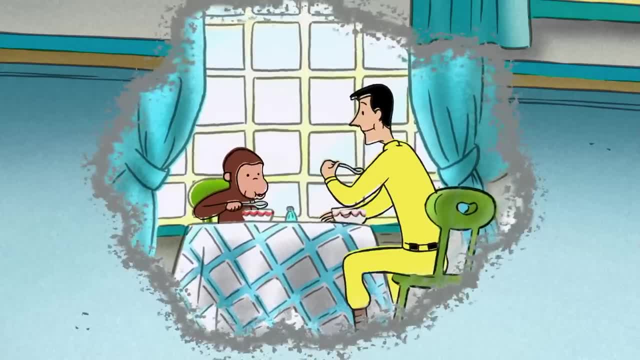 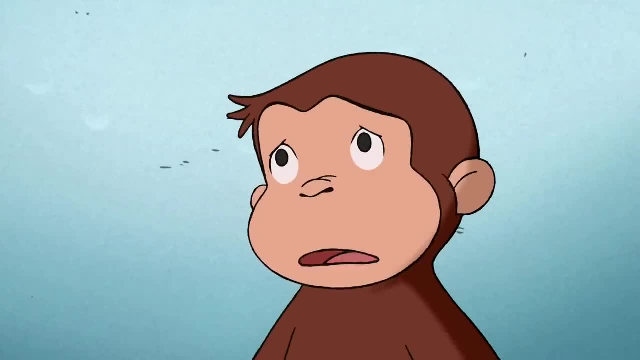 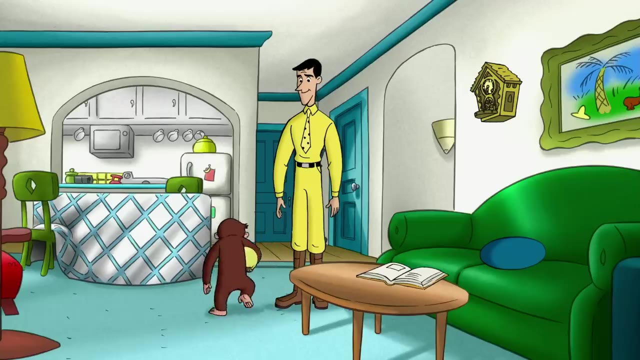 But now it's spring and the days are longer. It's light when you eat dinner and light when you go to bed. Hmm, Well, 7.30 means bedtime, no matter how light it is outside. George, Oh, I know. 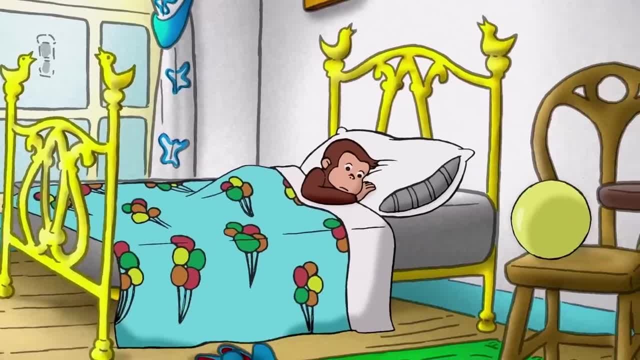 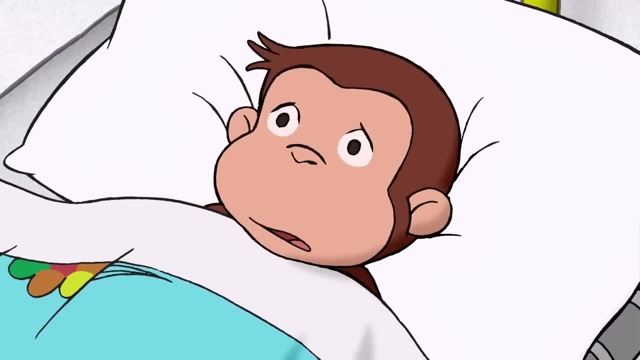 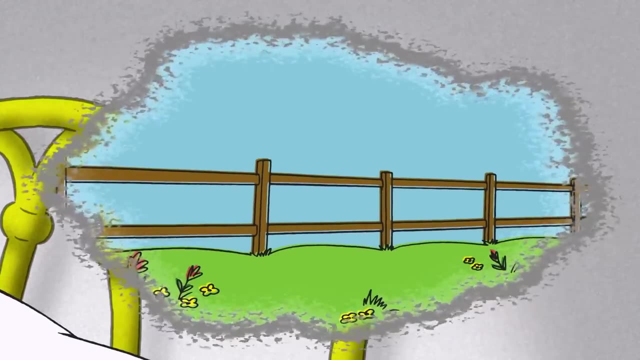 Oh, Oh, Oh, Oh Oh. It's hard to fall asleep with the sun out. Counting sheep seemed like a good idea. It's hard to fall asleep with the sun out. Counting sheep seemed like a good idea. Counting sheep seemed like a good idea. 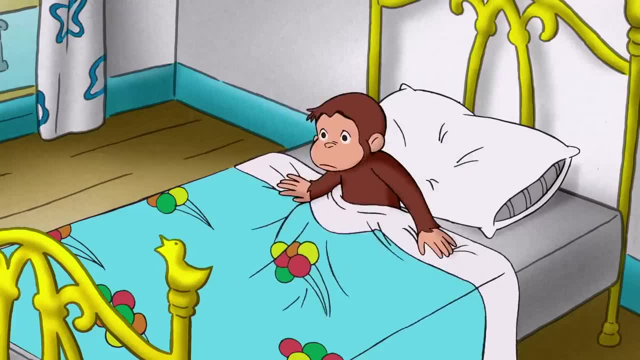 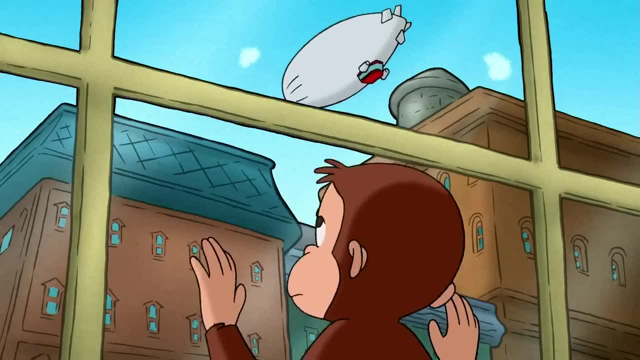 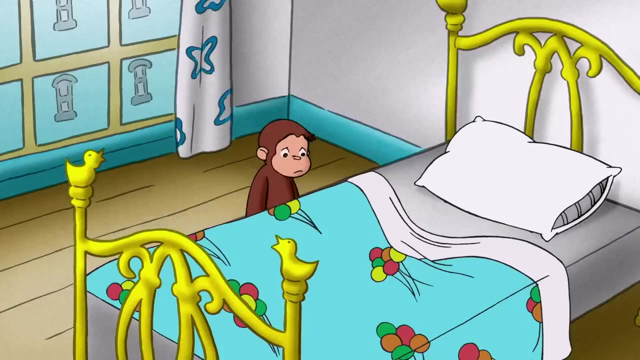 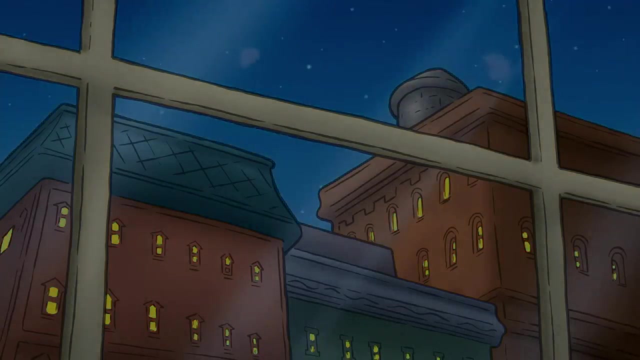 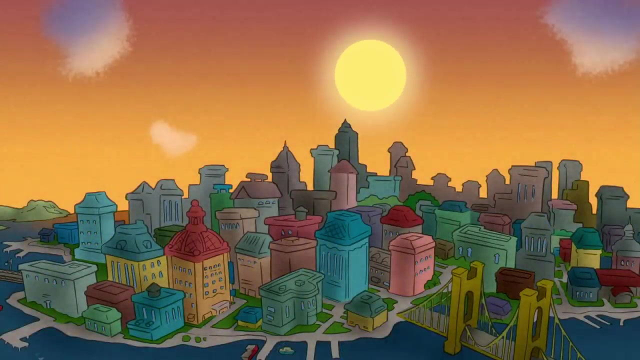 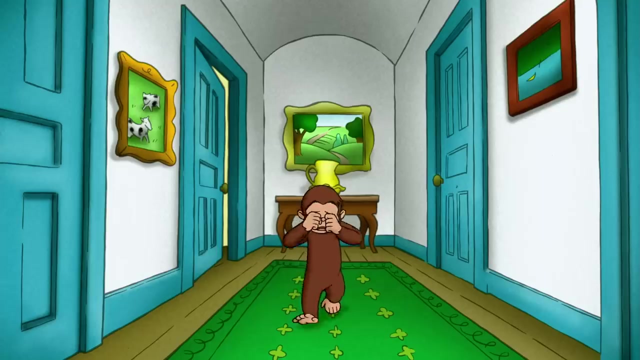 But even the sheep were out enjoying the sunshine. Ooh, Hmm, Hmm, Ooh, Ooh. It just wasn't fair to bed and miss all this. George didn't fall asleep until the sun went down. There we go. Good morning George. 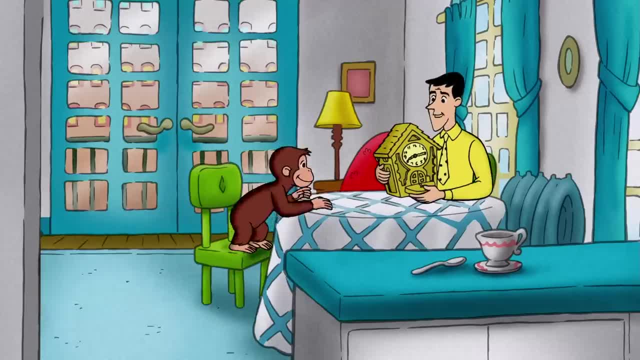 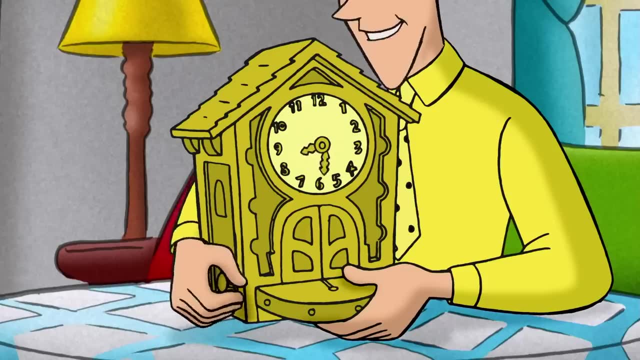 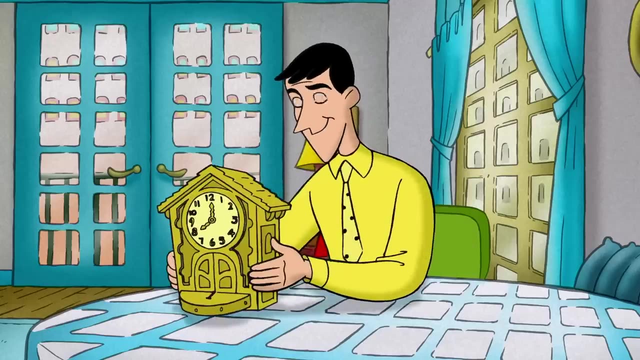 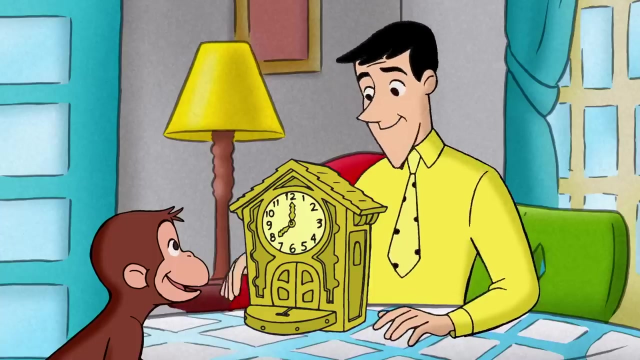 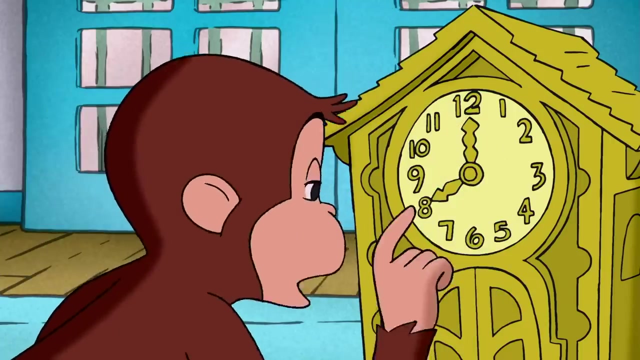 I put new batteries in the clock, so now I'm setting the time. Look, I can move the time forward, like this, Or backward, like this. See, the little hand points to the hour eight And the big hand tells you how long until the next hour. 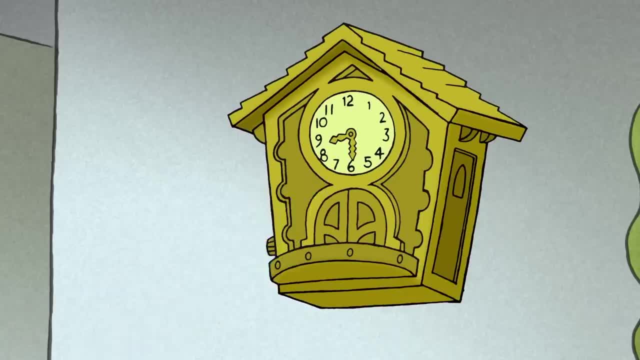 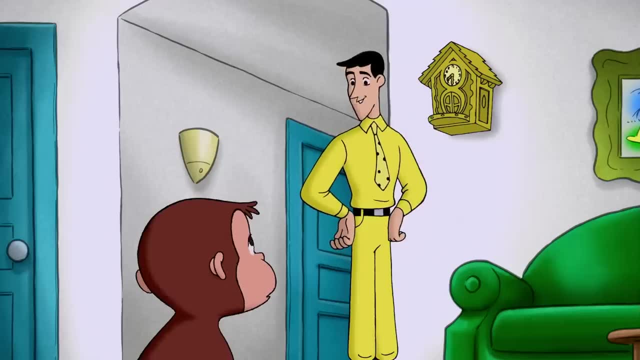 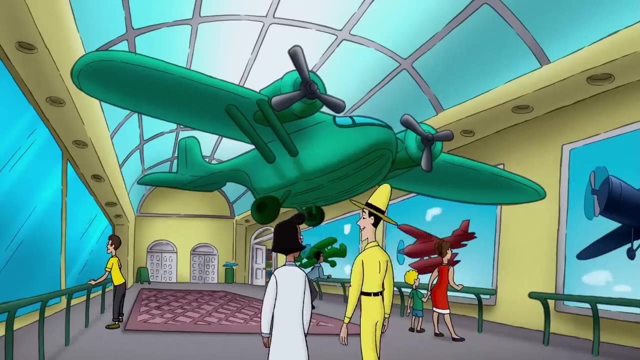 8.30. Halfway to nine o'clock. So while my bedroom clock and watch are in the shop, Olga will make sure we're on time for things like going to bed. You know, I'd like to get a surprise for George. 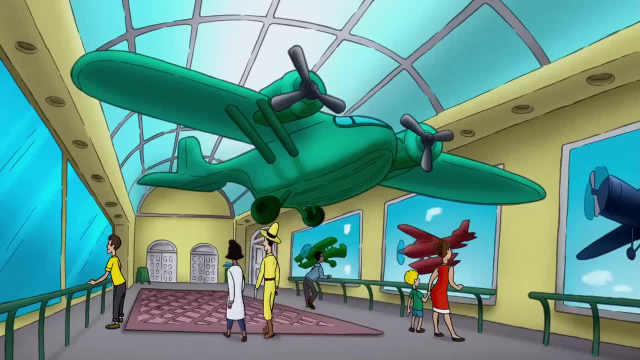 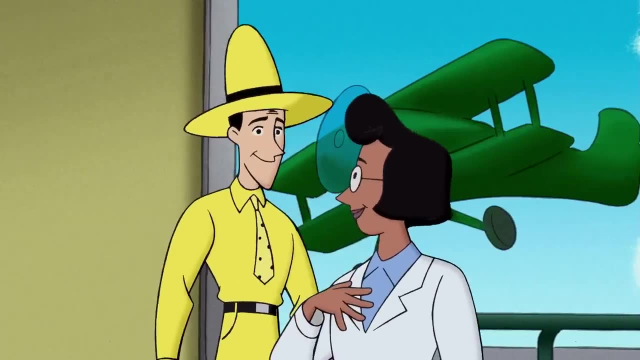 He's been really good about sticking to his bedtime. Hmm, Hey, what about a blimp ride? The Rough Week blimp is in town this week and I know the owner, Oh George, would love a blimp ride. Well good, Mr Rough Week will be here tomorrow at 9.30. 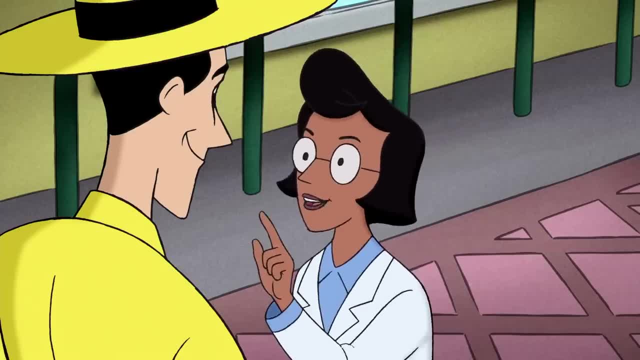 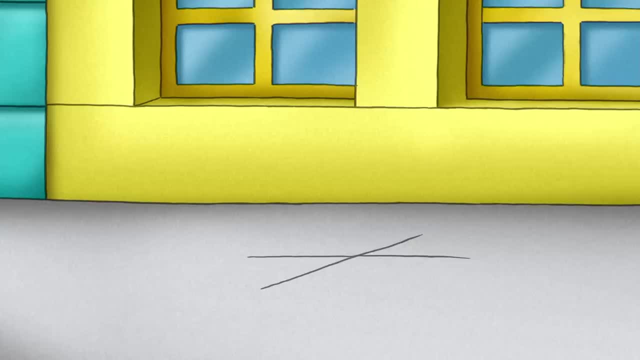 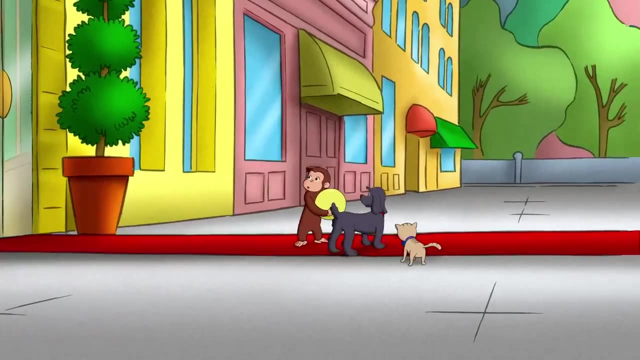 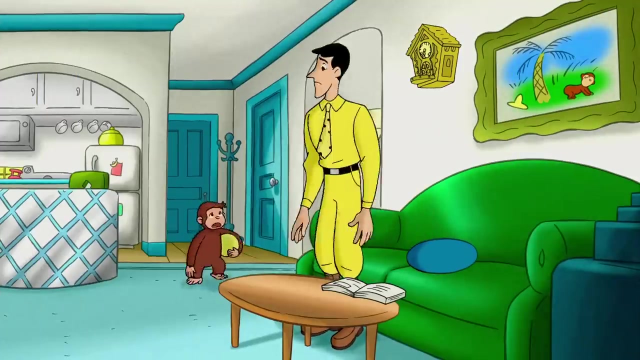 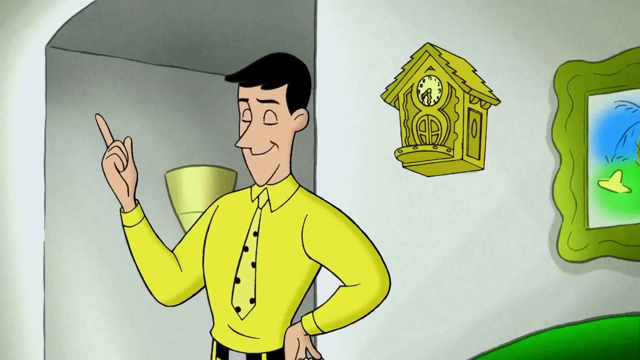 You can make an appointment with him, But be on time. Mr Rough Week keeps a tight schedule, George, it's bedtime. I'm sorry, George, It's 7.30.. If it were 6.30, you could keep playing, but it's not. 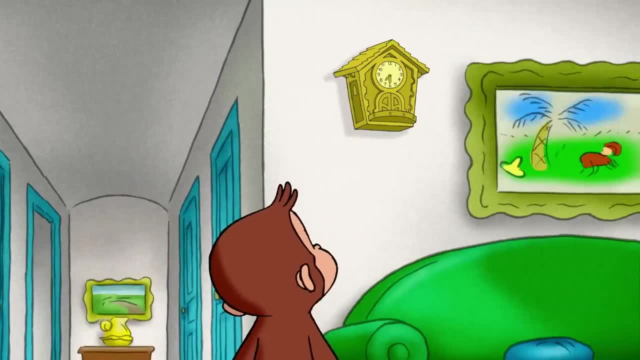 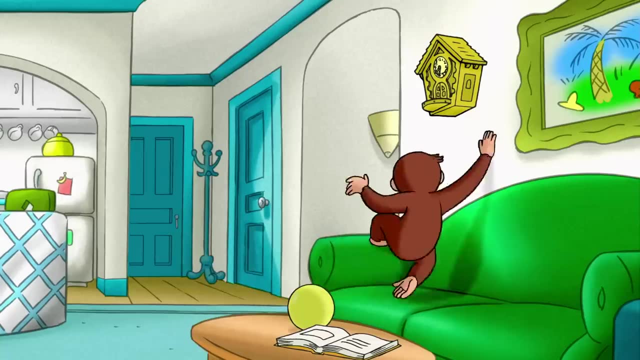 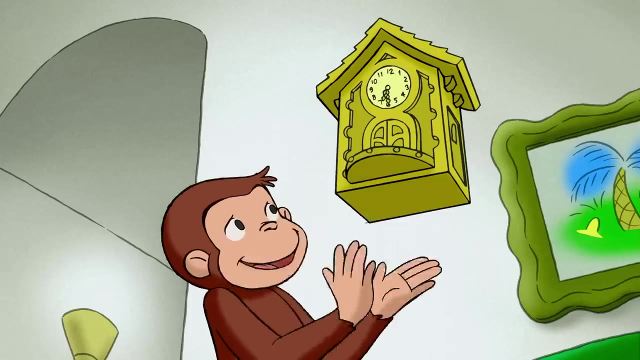 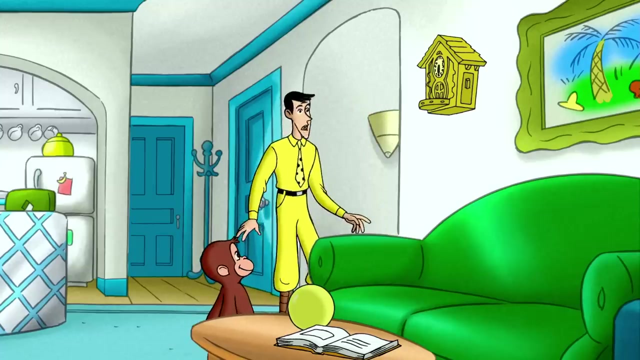 6.30?. George just learned how to change time this morning. Ah, Ah, Ah, Ah, Ah, Ooh. Well, your bed is all ready for you. Ha, ha, ha, Oh, it's only—. Huh, I thought…. 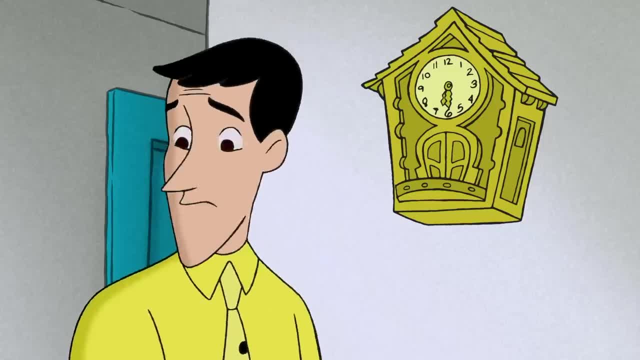 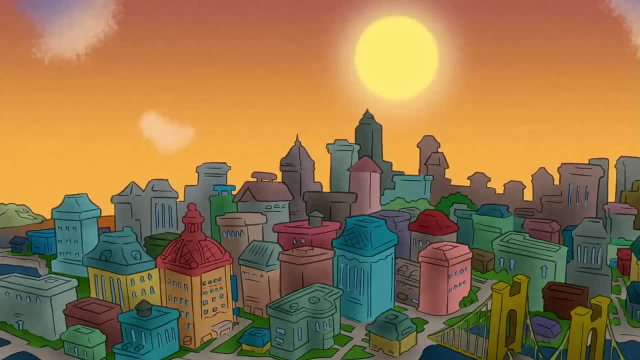 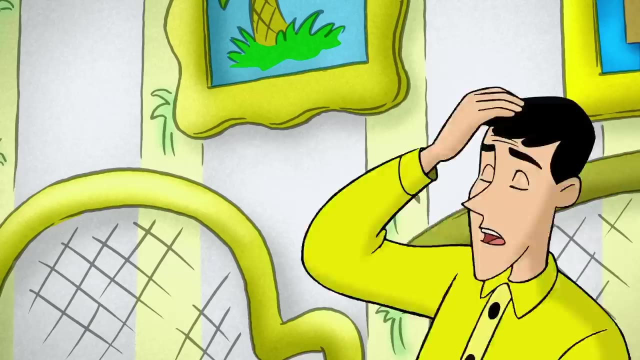 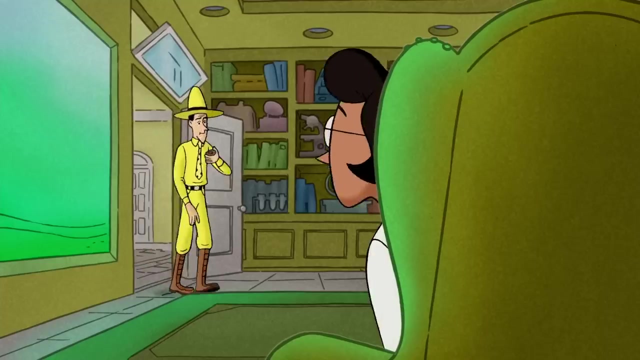 Oh, sorry, I guess you still have an hour to play. Yay, Hoo, hoo, hoo, Ha, ha, ha, Ha, ha ha. Oh, can't be late. What happened? Well, they were out of jelly donuts, so I got chocolate. 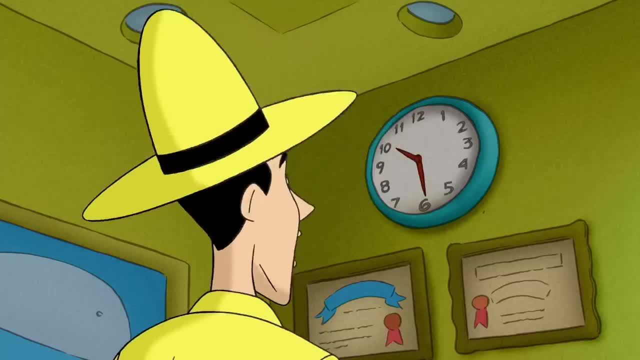 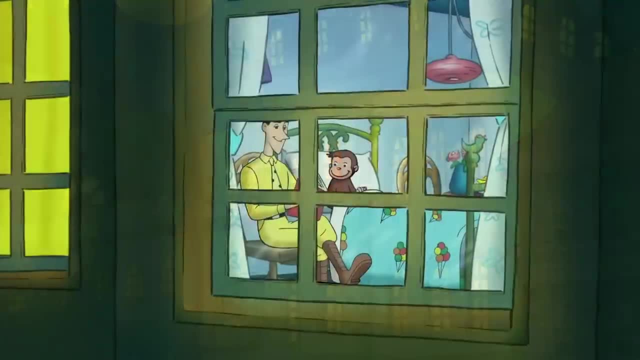 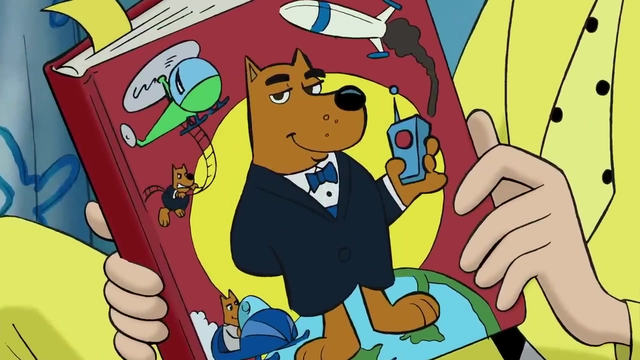 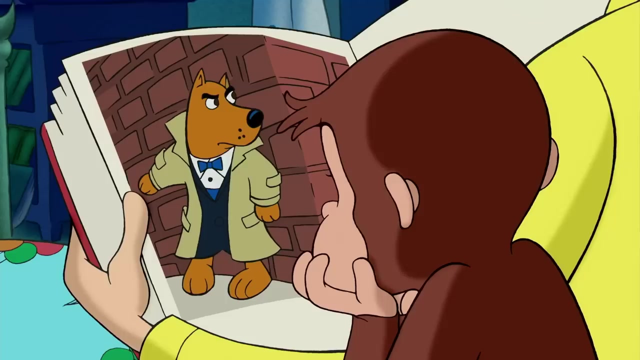 You're late, I, I, I. that's not possible Bedtime in the city, When all little monkeys like to hear a good story. Of all the bedtime stories, Double-O-Doggy was George's favorite. It's a super spy's job to discover secrets and Double-O-Doggy is the best. 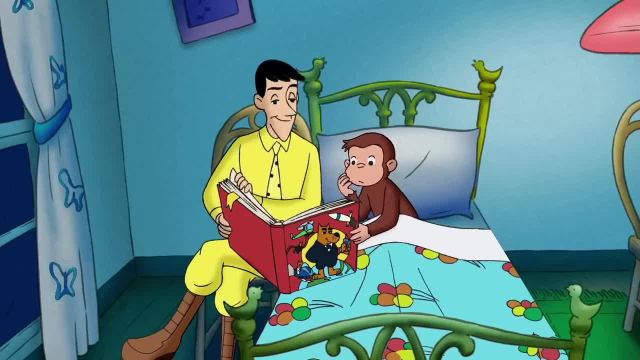 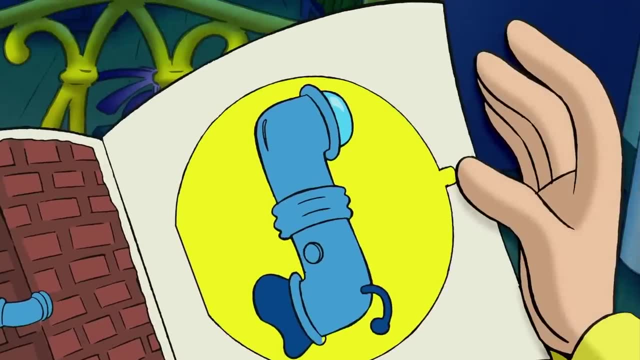 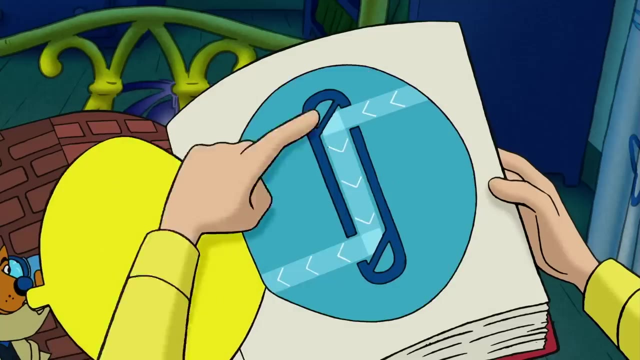 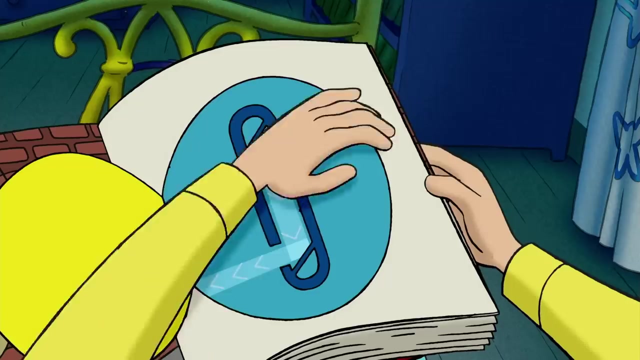 He has lots of tools to help him. Well, that's a periscope, remember? Well, inside the tube are two mirrors. The mirror at this end reflects whatever it's pointing at to a mirror at this end. That way, Double-O-Doggy can see things without being seen himself. 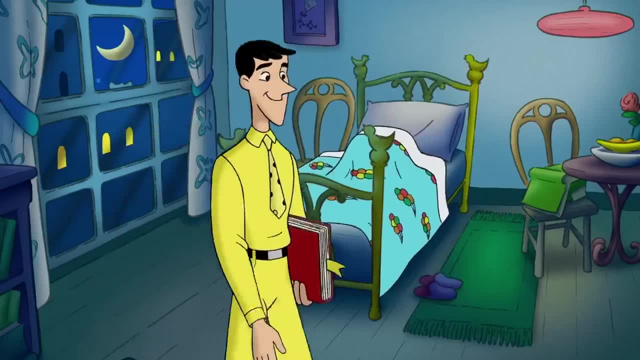 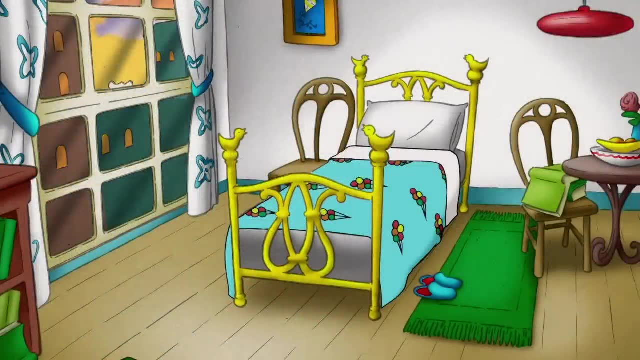 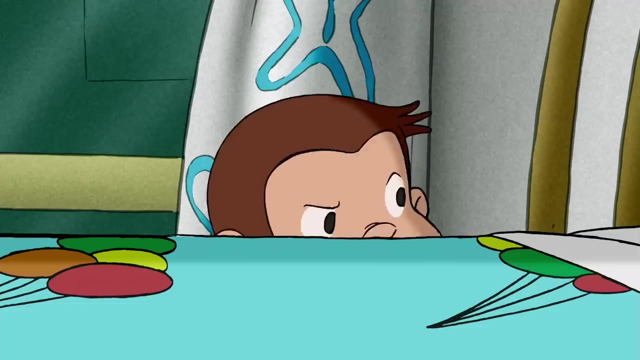 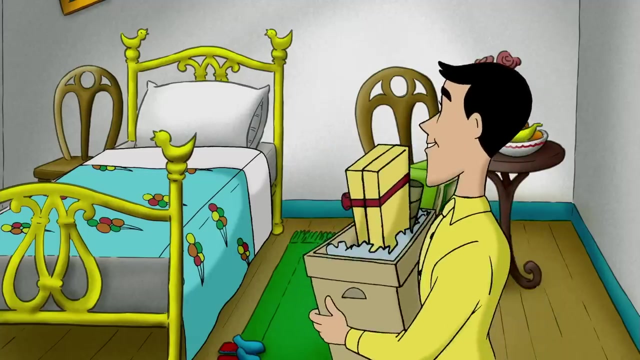 All right, good night, little spy monkey. The next day, George started practicing to be a super spy like Double-O-Doggy George, if you have any paper to recycle, put it in this bin, okay, Um, George. 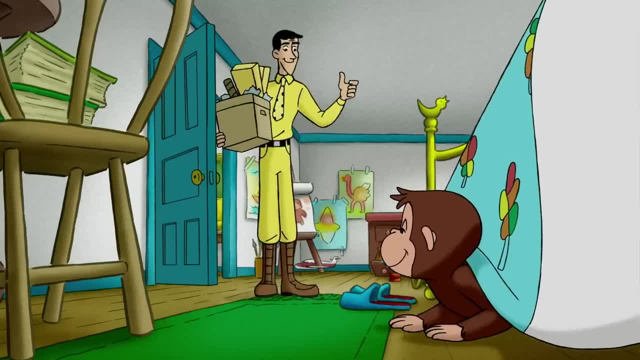 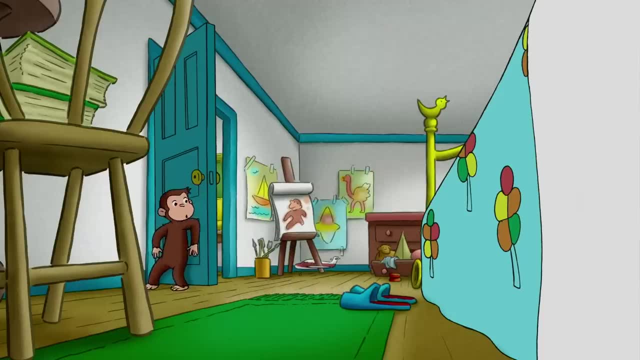 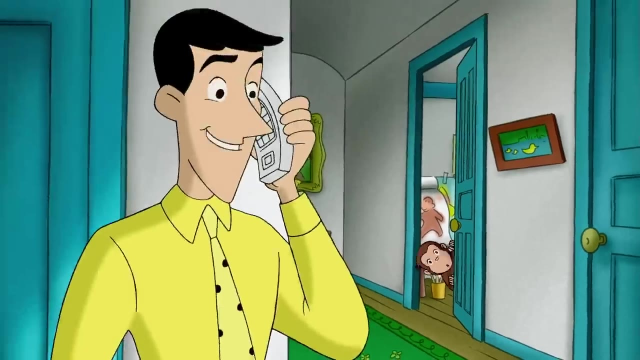 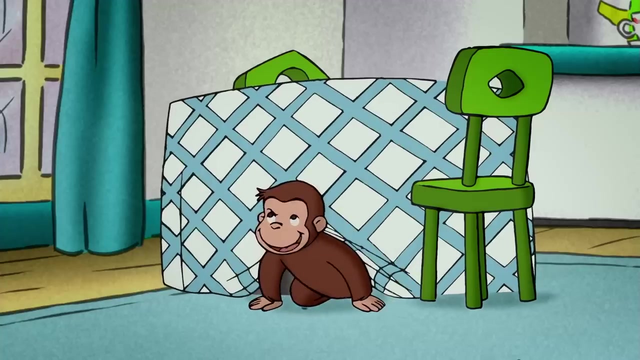 Woo-ha, Woo-ha. A super spy needed a spy name. George became Double-O-Monkey Professor Wiseman. I was wondering: Can we meet? an hour later, A super spy had to be smart, quiet and quick with his hands. 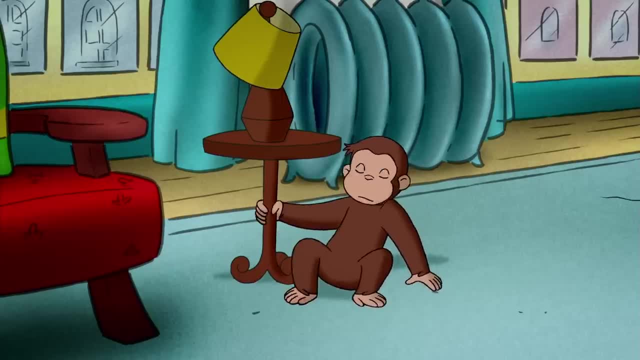 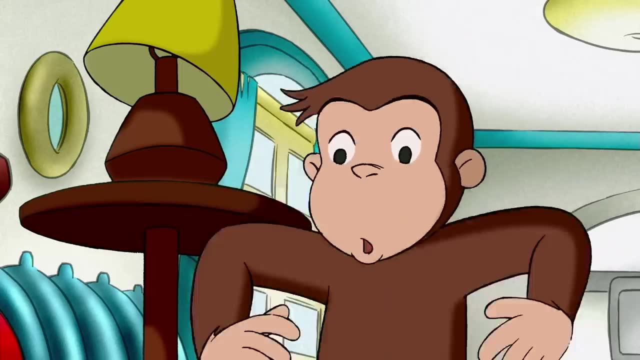 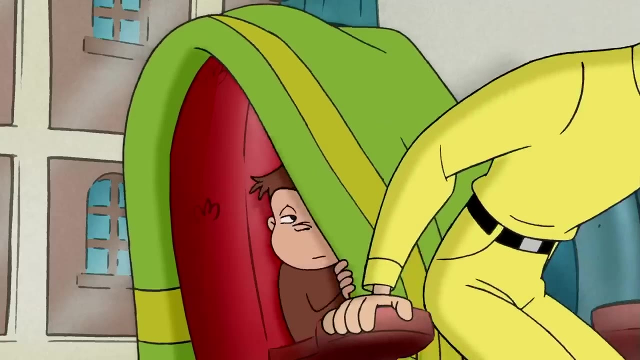 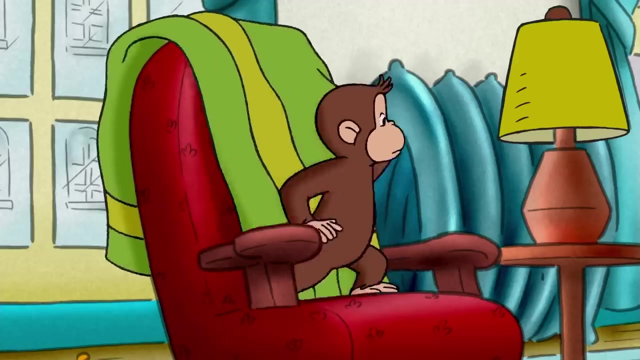 And feet. There's this thing I want to get for George. He is going to love it. Sometimes super spies had to go undercover. Oh great, See you. then. He'd only been a super spy for two minutes and Double-O-Monkey already had his first spy mission. 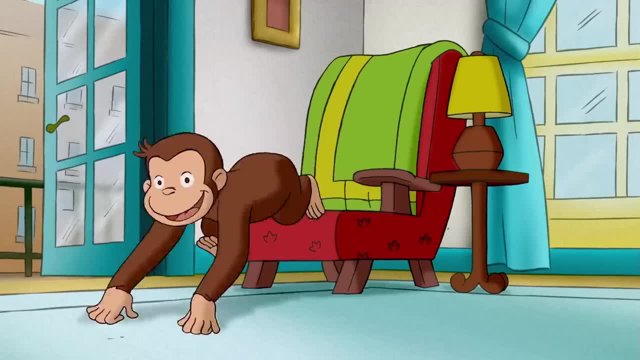 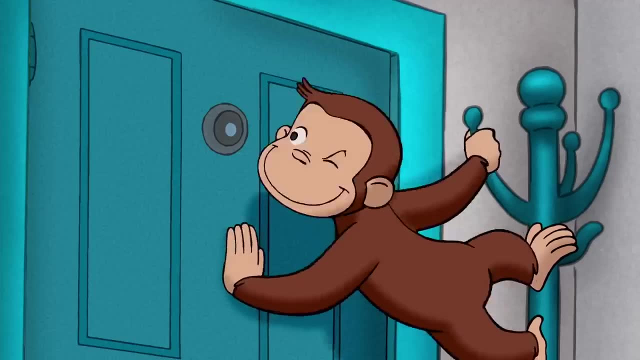 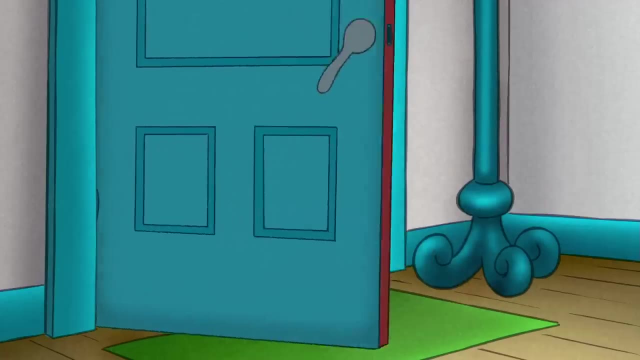 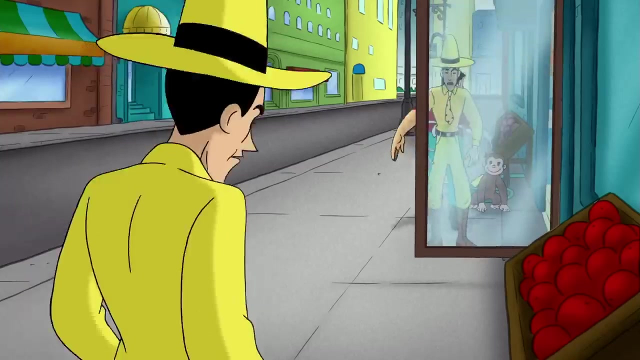 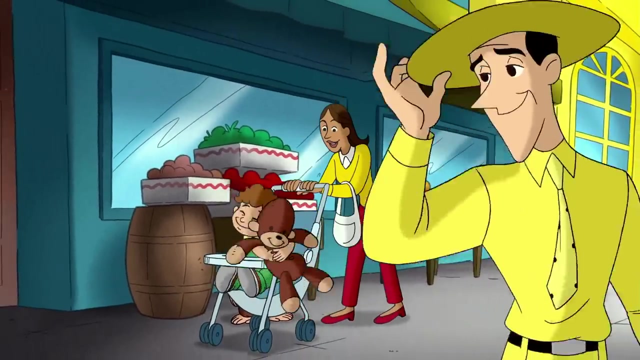 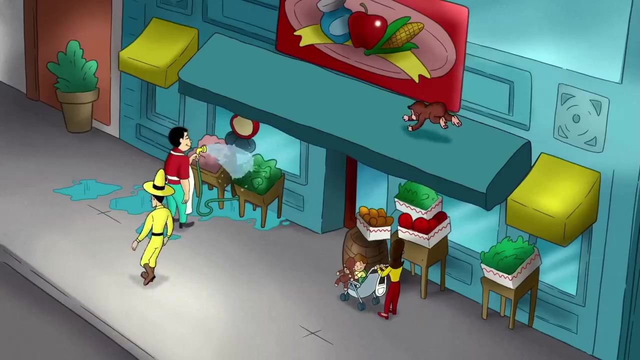 Find out what the man with the yellow hat was going to get him, But he had to make sure he wouldn't be seen. Woo-ha-ha, George, George, Staying out of sight was complicated. Hi, how you doing. 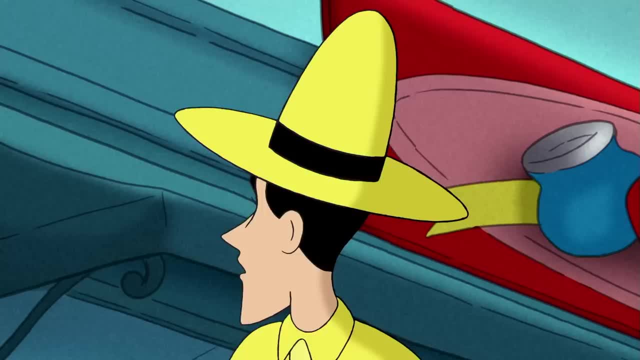 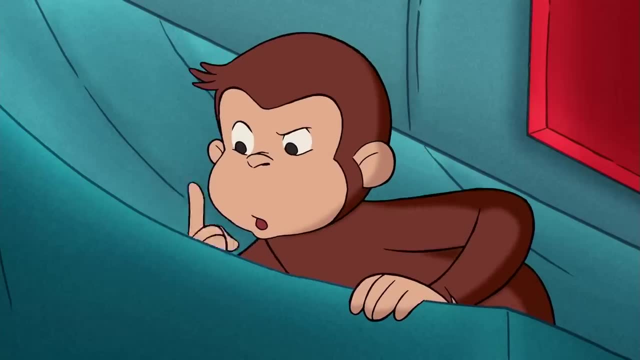 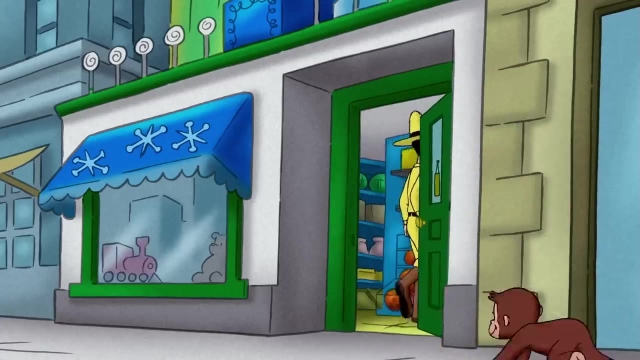 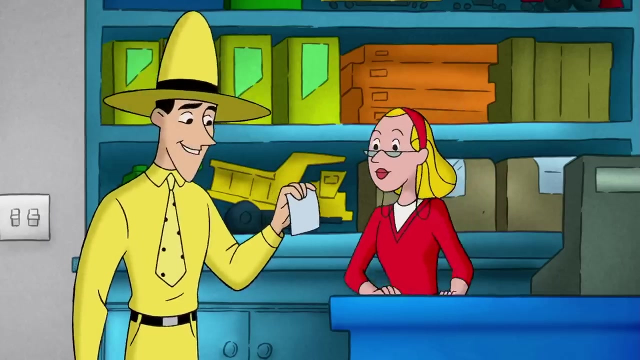 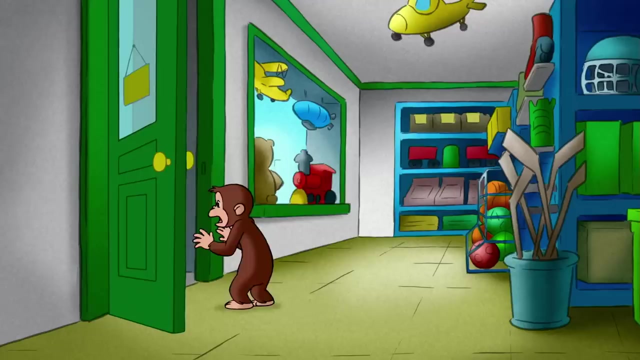 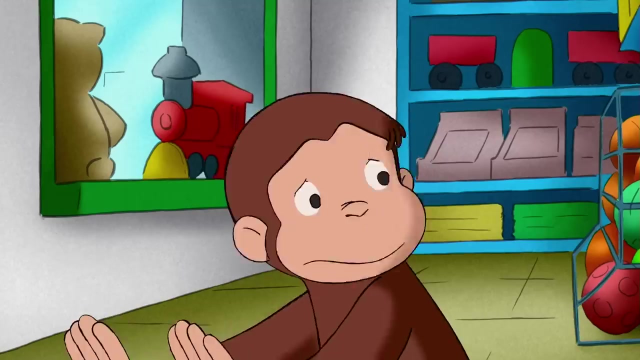 What, George? Hmm, No, Even puddles could give you away. Do you have this in stock? A barking charky was even worse than a puddle Shh. The last thing a spy wants is to attract attention. 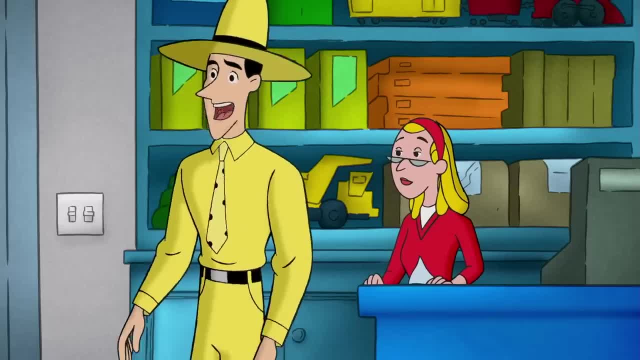 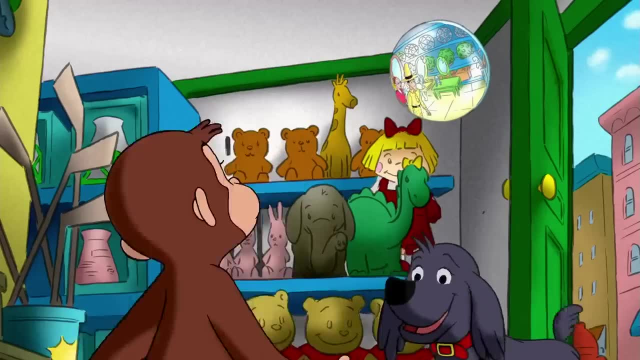 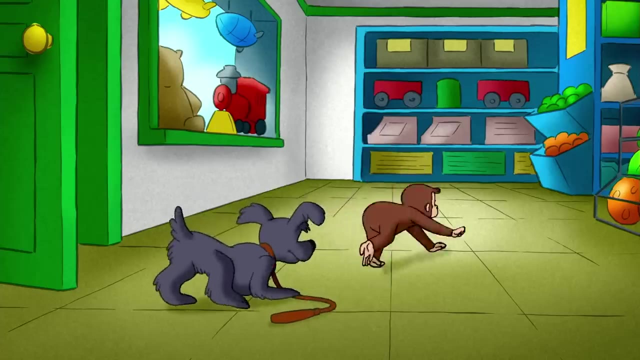 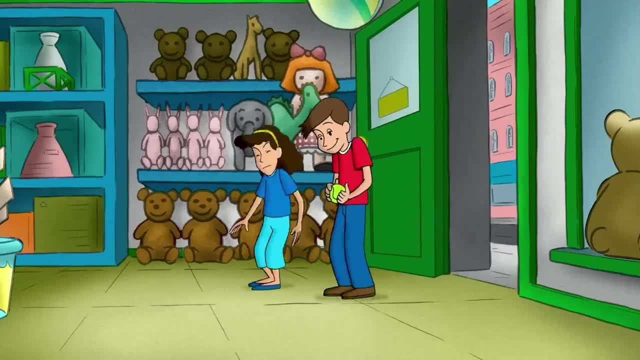 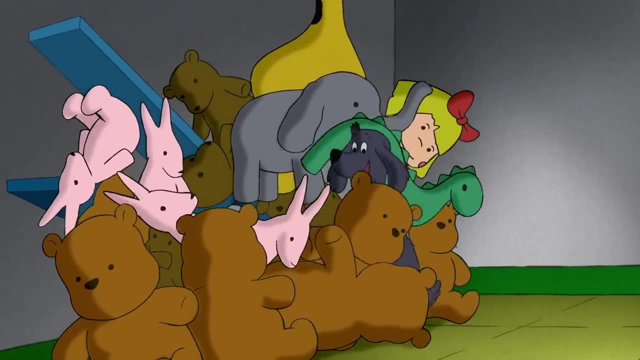 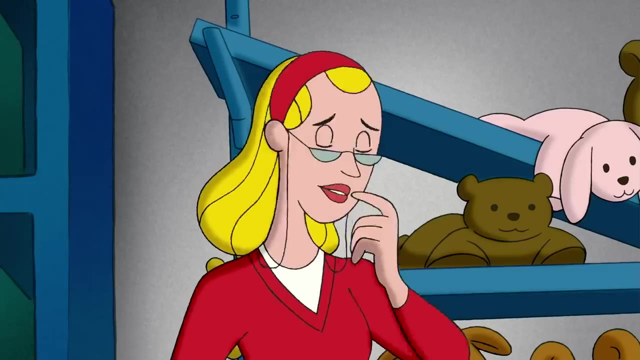 Woof, I got it. Woof, woof, woof, woof. Oh Well, we found charky: Woof, woof, woof, woof. Sorry, We'll help clean that up. No, it's all right. 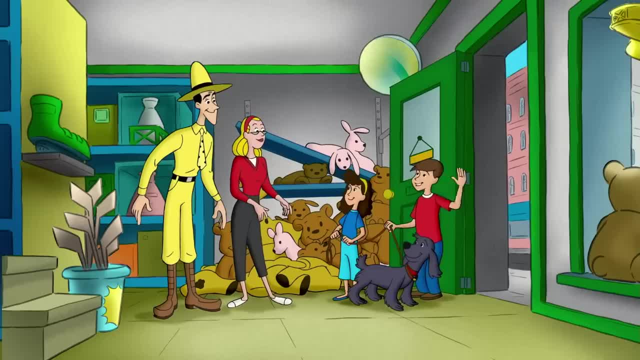 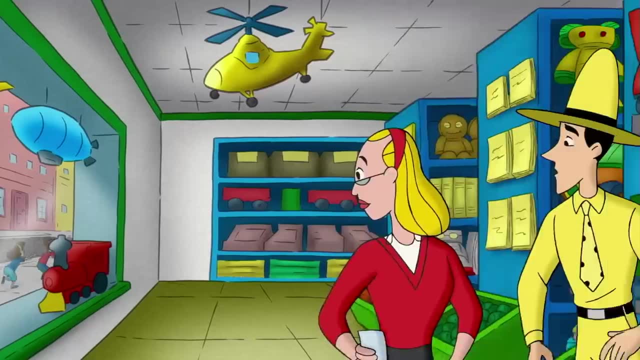 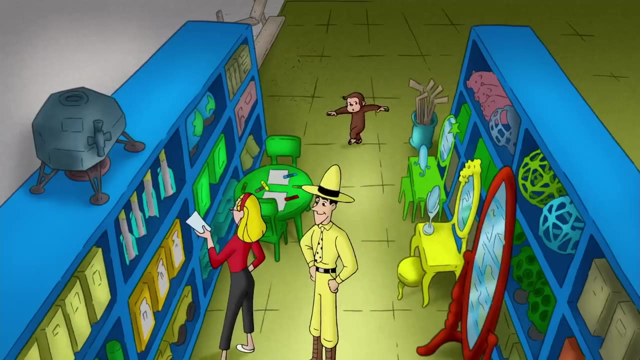 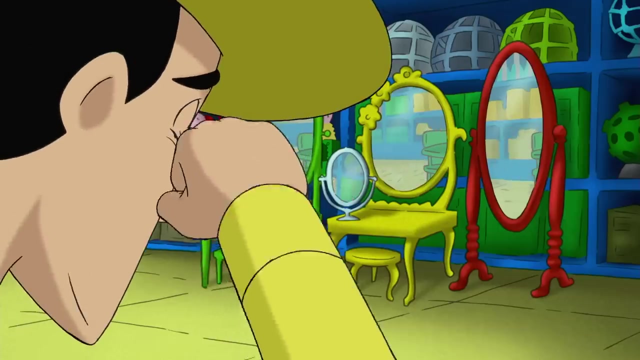 Just take charky, home. Thanks, Okay, bye, Woof, Woof, woof, woof, woof. Hmm, Let's see, now It should be here, somewhere, Here, Aaaah, Woof George. 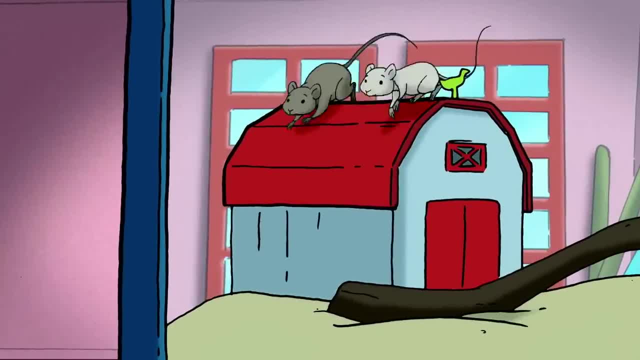 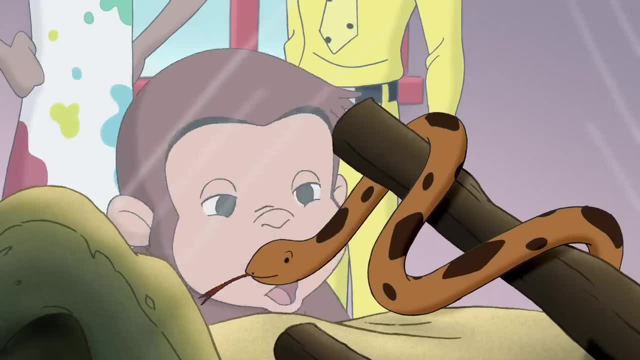 Benji and Willy were George's favorite mice in the entire world And Bruno was the only gopher snake he knew personally. So when Mr Zubel asked him to pet-sit for him, he said: And Bruno was the only gopher snake he knew personally. So when Mr Zubel asked him to pet-sit for him, he said: 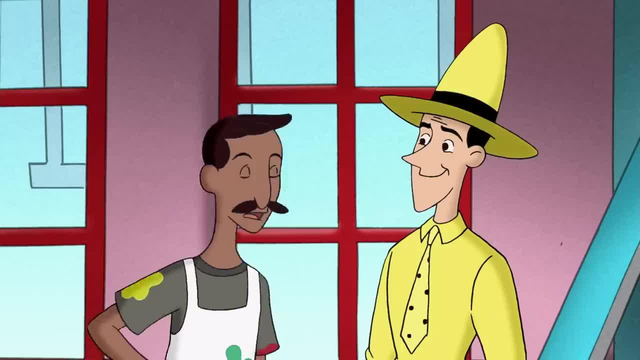 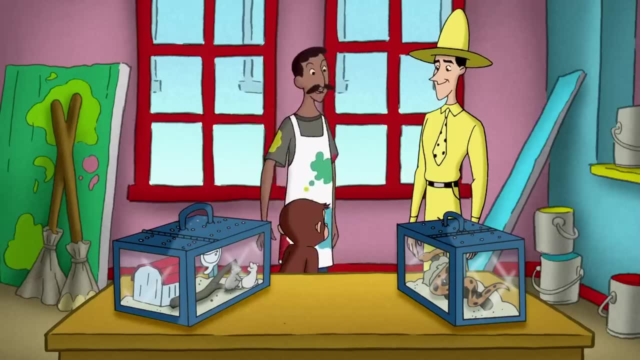 So when Mr Zubel asked him to pet-sit for him, he said: for a day, George was thrilled. Thanks for helping me on such short notice, George. I have to be at the zoo morning till night studying feet for my new mural. 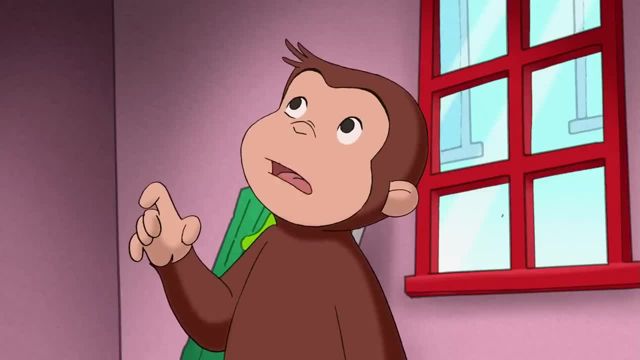 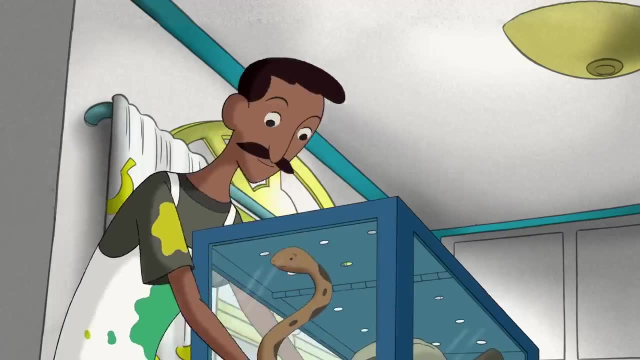 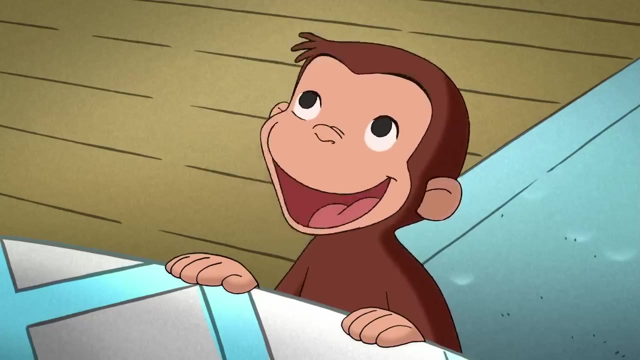 Rhino, What You Did Last Summer. Now Bruno has already eaten an egg, so he won't be hungry anymore today. Don't feed him. The mice must be fed, but I'm out of food, So I told the pet shop you'd be coming by. 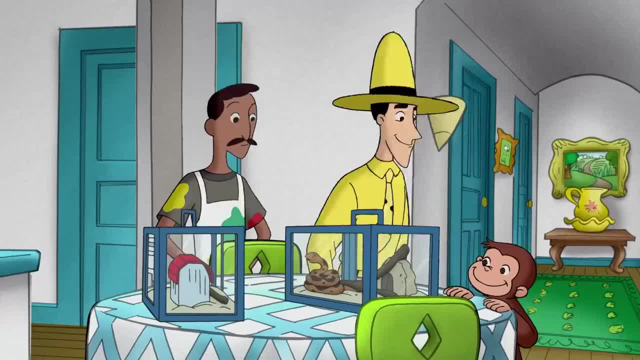 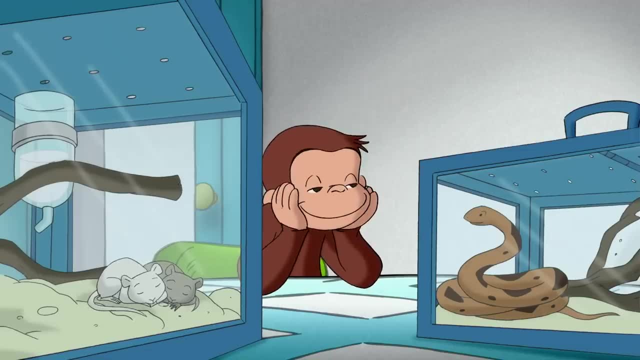 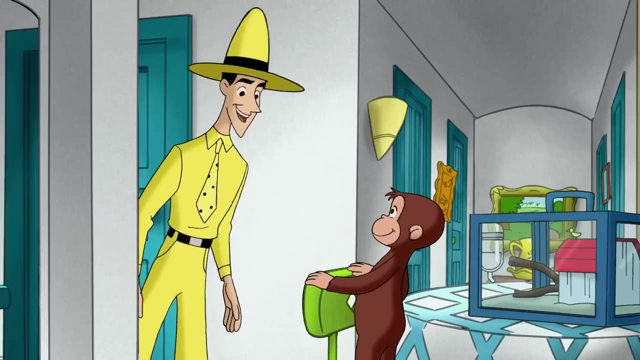 to pick up mouse food. George was determined to be the best pet sitter ever, So he sat. See you tonight. Thanks again, George. I have to go talk to the park director about Heritage Week. Will you be okay by yourself? 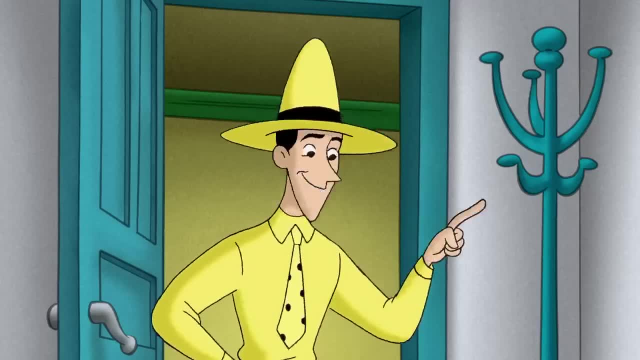 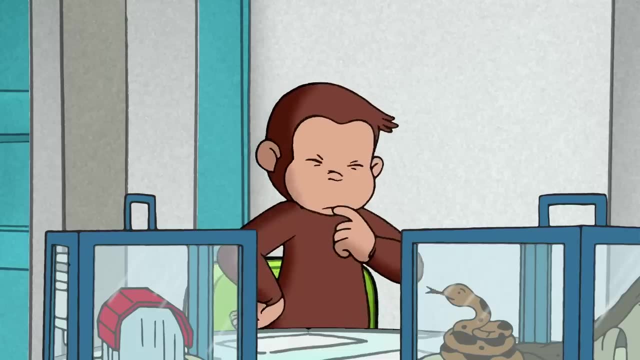 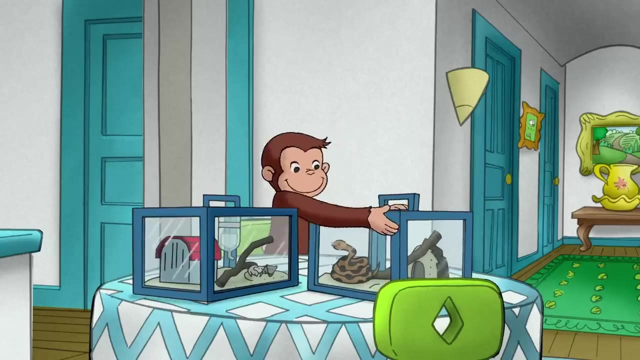 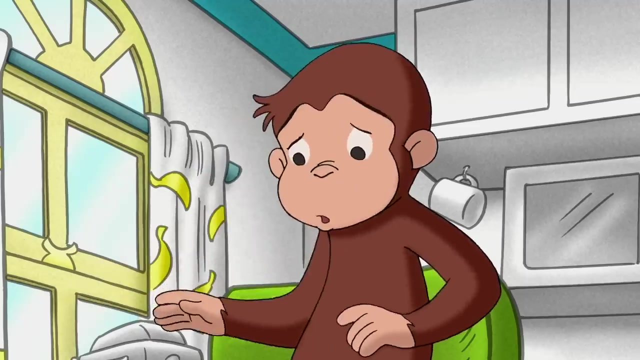 Be a good little monkey pet sitter. A good sitter makes his siti feel at home. Since these guys lived together, they were probably used to being closer together. They didn't seem happy about that. Ooh, Ooh, Ooh. 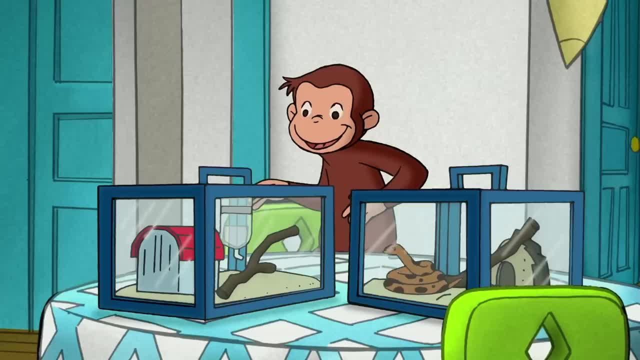 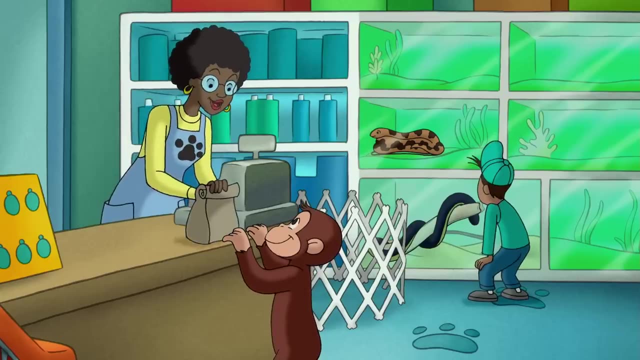 Ha-ha. Of course they weren't happy. They were hungry. Time to get food. Hoo-hoo-ha-ha, Ha-ha-ha-ha, Here you go. One bag of mouse treats for Benji and Willy Zuvel. 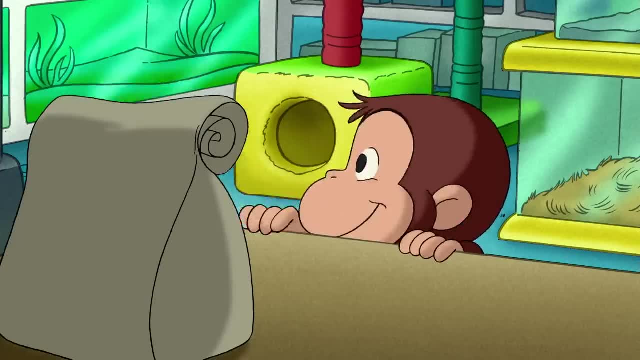 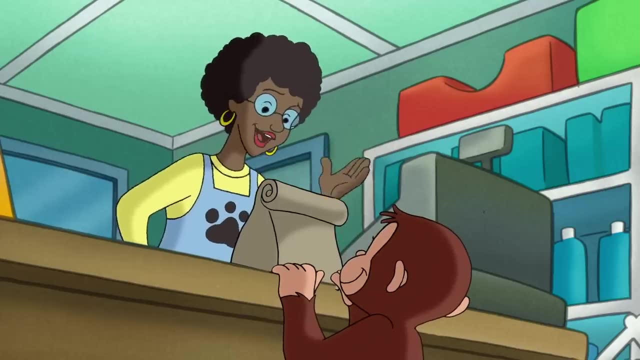 Ha-ha-ha-ha. Excuse me, Would I have to feed a snake long skinny food? No, Snakes eat fish. Insects bite Baiters, mice- Yeah, Mice. earthworms slugs eggs. 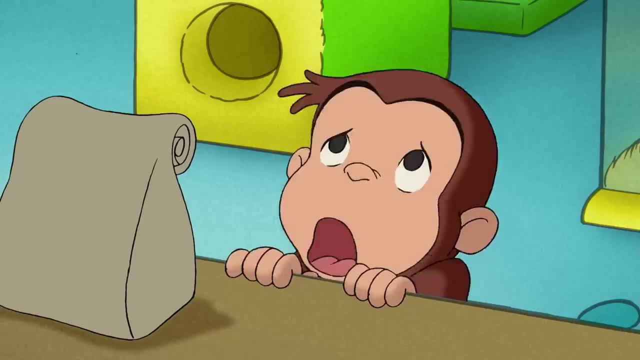 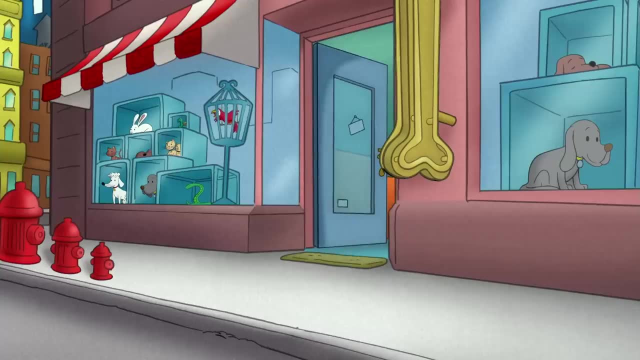 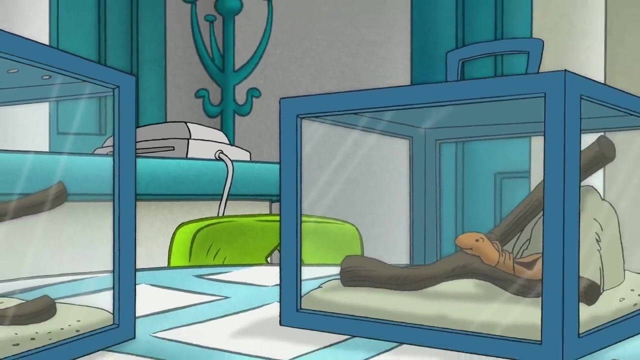 And they only eat once a week, Sometimes once a month. No wonder Benji and Willy didn't want to be near Bruno. Ah, Ow, ow, ow, ow, ow, ow, You forgot your mouse food. Hola, Zuvel here. 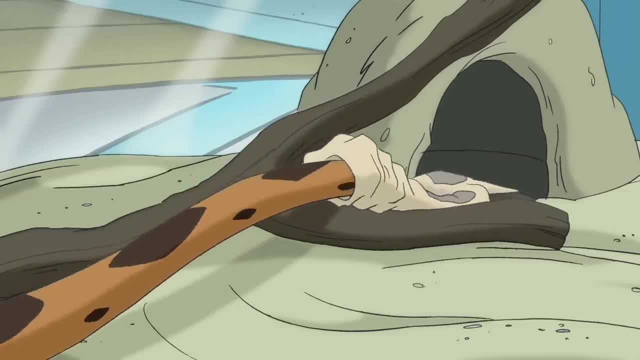 I didn't tell George that Bruno is about to shed his skin. He only sheds three times a week. He only sheds three times a week. He only sheds three times a week, Three times a year. He only sheds three times a week. 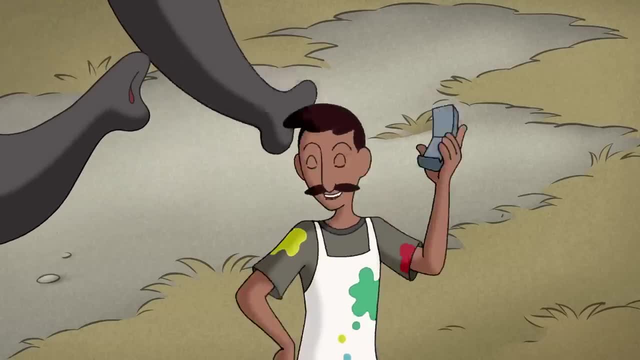 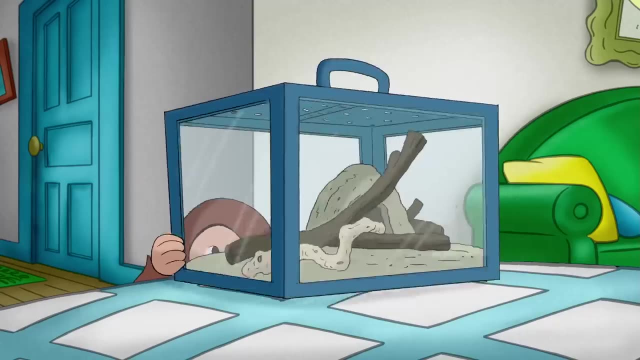 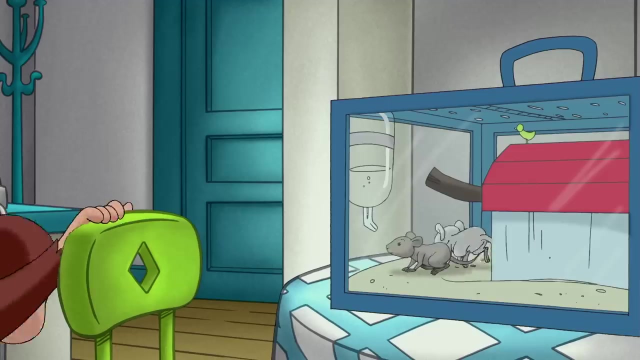 He only sheds three times a week. So watch for it, So, watch for it. It's worth seeing. Sorry, I'm out of peanuts, Ha ha ha. George reassured the mice that they were safe the whole time. George reassured the mice that they were safe the whole time. 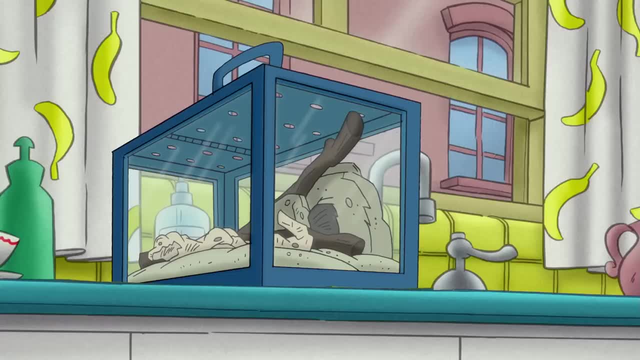 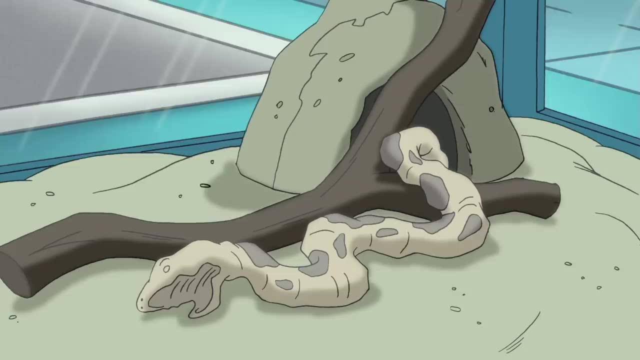 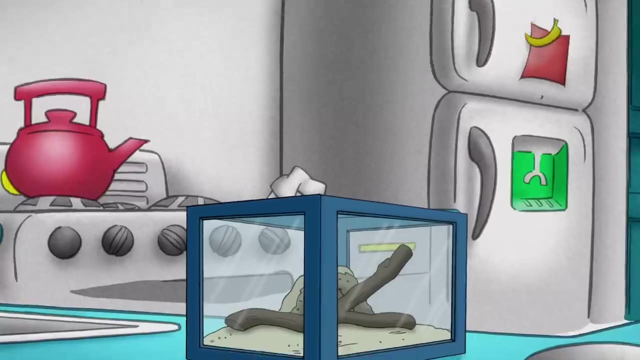 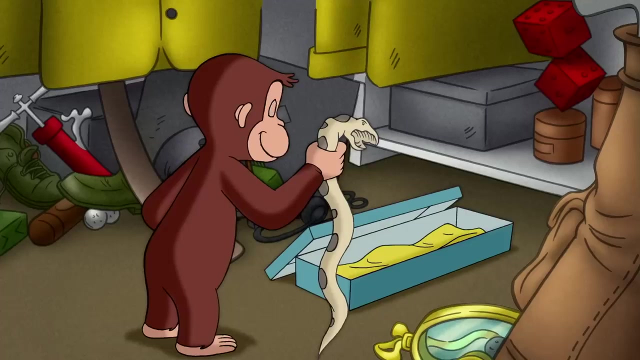 Ha. When he went to make sure Bruno liked his new spot by the window, Ha Ooh Ooh, He noticed Bruno had changed. What happened to him? The pet shop owner knew all about snakes. George could bring Bruno and ask him. 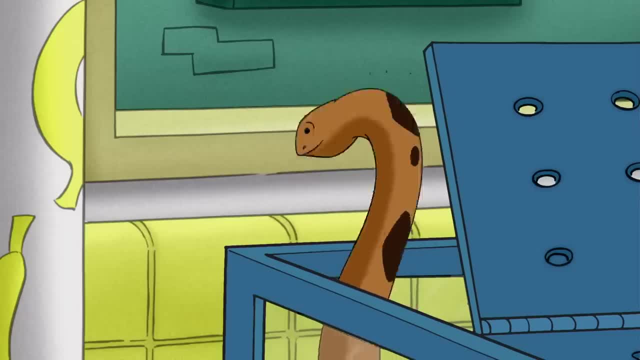 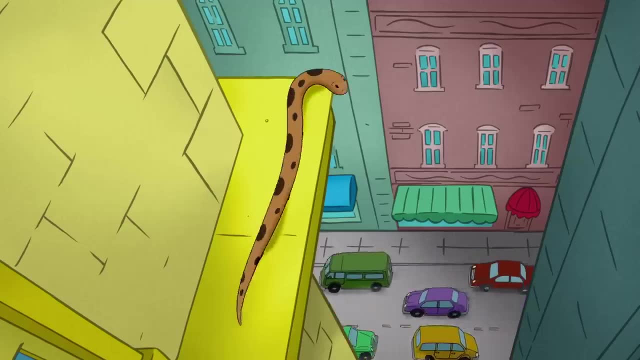 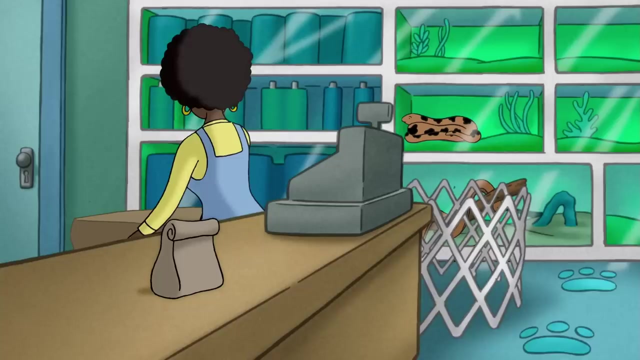 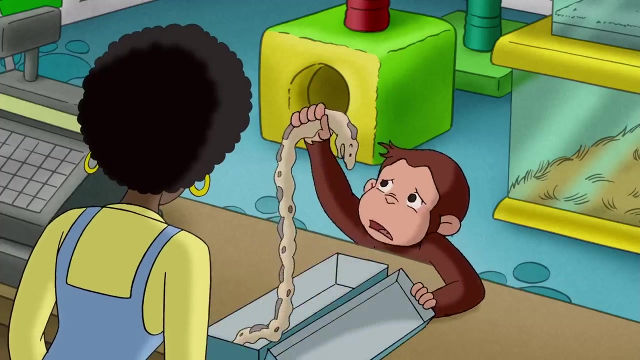 Like any snake. when Bruno saw that warm sun, he wanted to be in it. The sun was warm, but city life was too noisy for a snake. He wanted to find somewhere quiet. Came back for this. Ah, I see Bruno shed his skin. 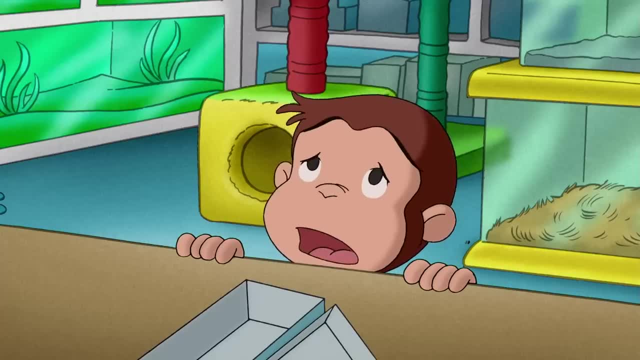 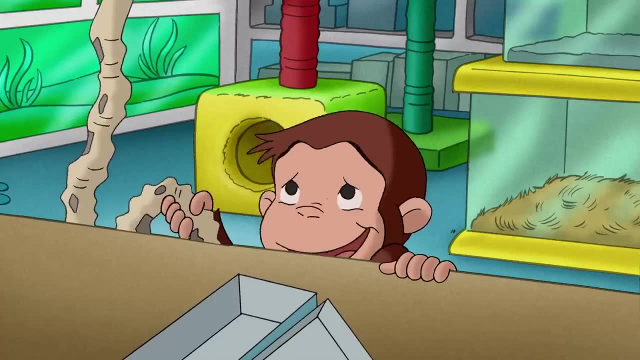 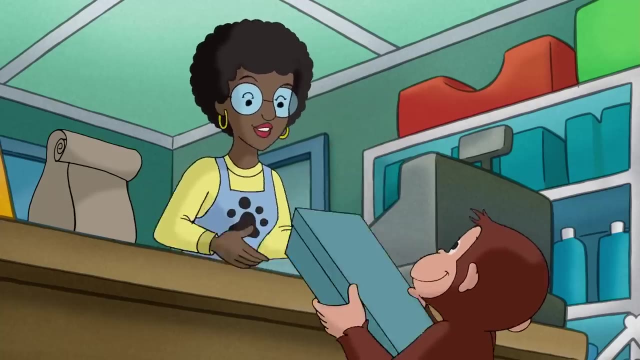 Mr Zubo was waiting for it. As a snake grows up, it wriggles out of its mouth This old skin. Did you think this was Bruno? I'll bet Bruno is under his rock. That's where he always goes after his sheds. 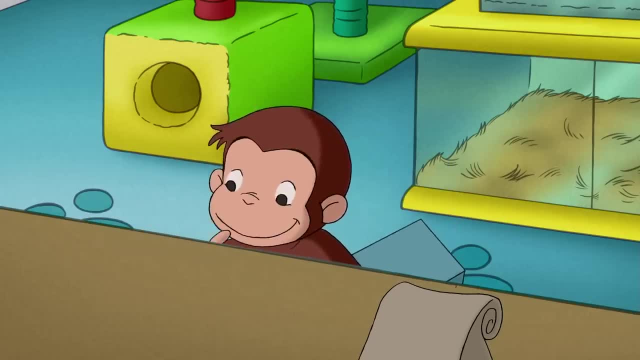 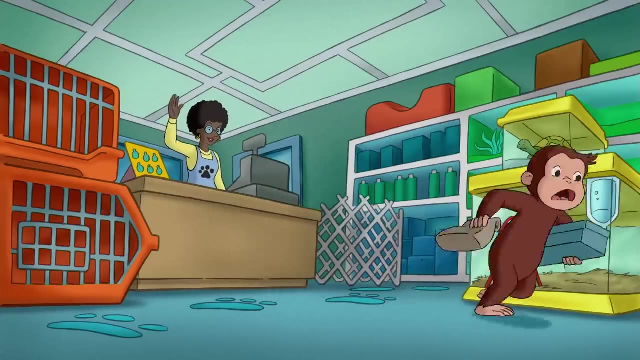 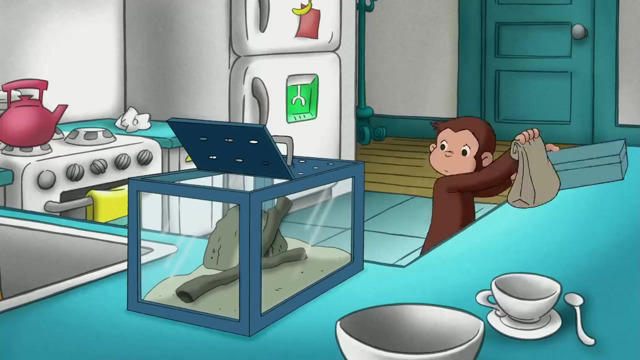 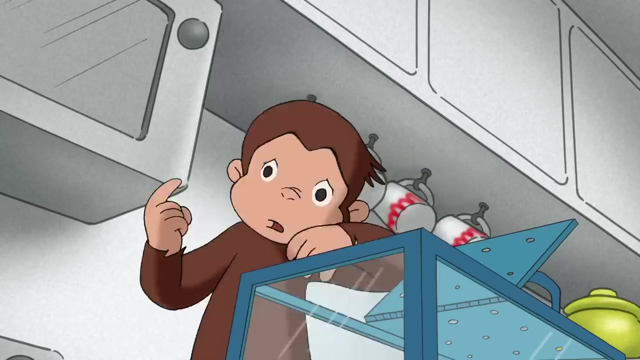 George was relieved to hear Bruno would be safe in his animal habitat, Until he remembered he left the habitat open. Bruno must have crawled out. He was in a state of shock.